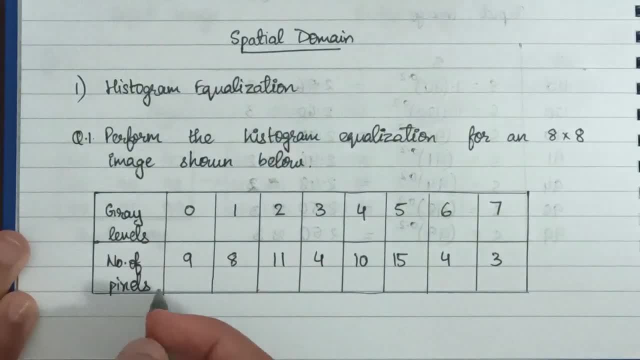 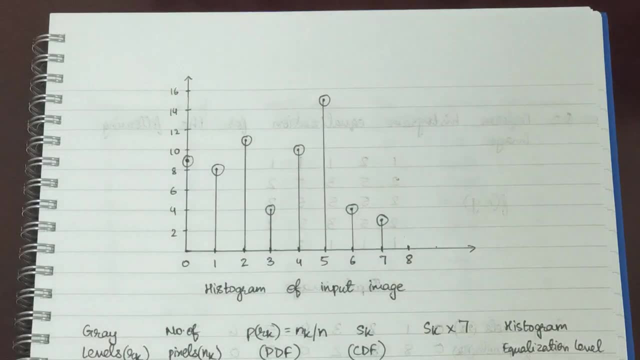 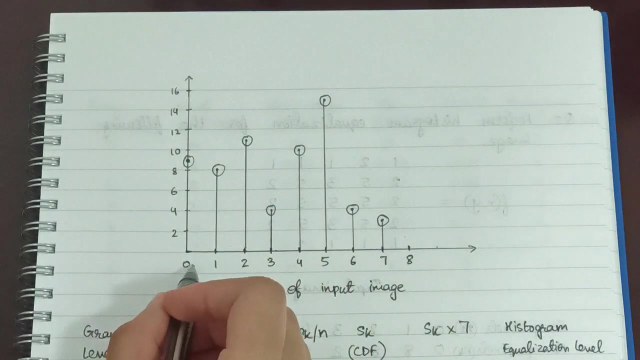 okay, and we have the frequencies or number of pixels for each of them. Now, based on the above table, we can draw this histogram of input image here, okay, where all of these 0,, 1,, 2,, 3, all of these represent the gray levels and these 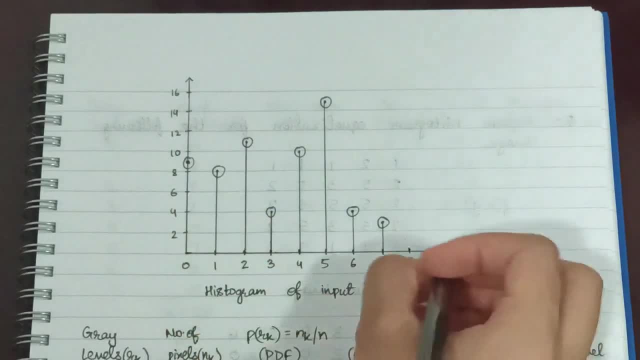 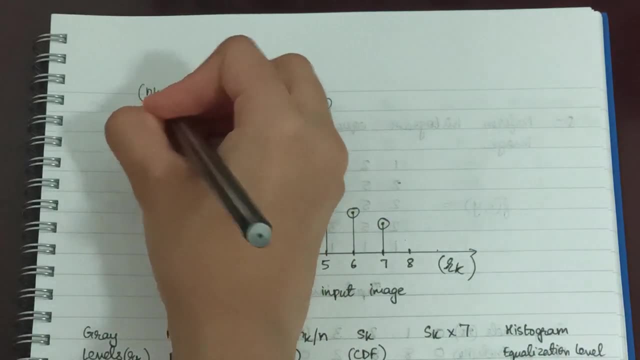 represent the gray levels. So we can draw this histogram of input image here, okay, where all of these- 0,, 1,, 2, 3- all of these represent the number of pixels. So the x-axis represents the gray level and the y-axis represents the number of pixels. So you can see for 0 we have the value. 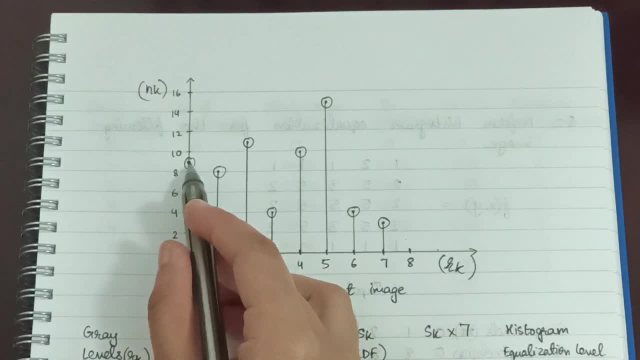 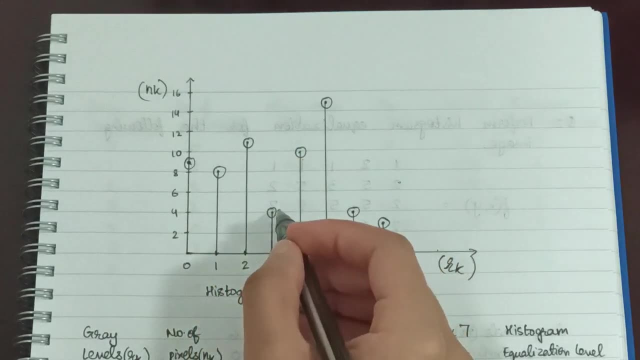 9- okay, which was given in the previous table. and similarly, for 1 we have the value 8, for 2 it is 11, for 3 it is 4 and so on. So we have marked each of these gray levels and their 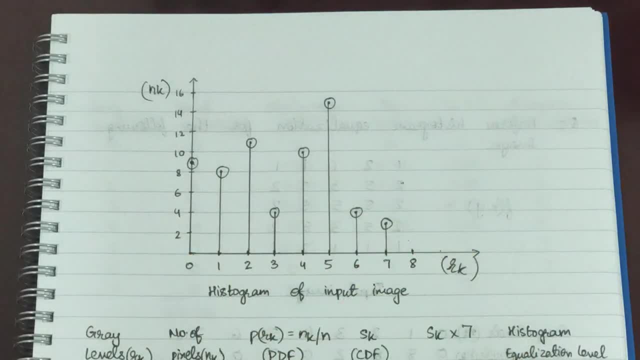 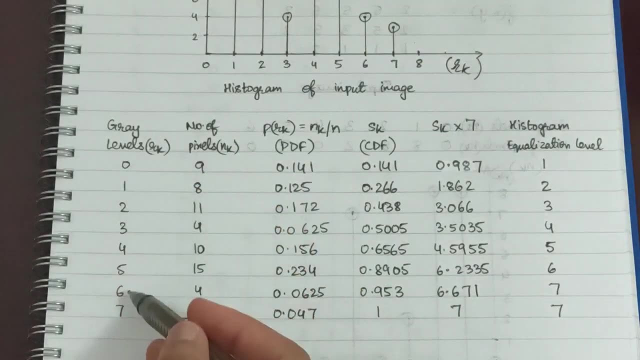 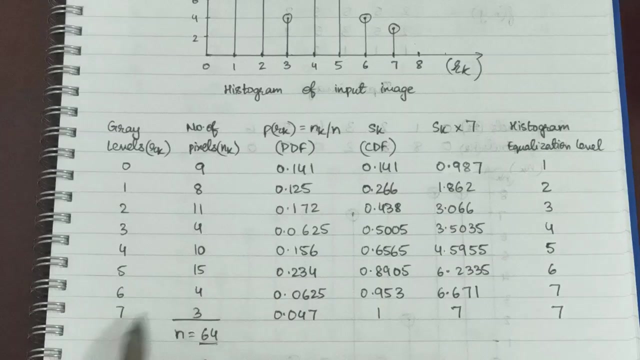 number of pixels in this histogram here. Next, we are forming the table here, The gray level values and the number of pixels. we have just written it down from the question. okay, each of these values we have written it down and now we will calculate the probability distribution function. So this is. 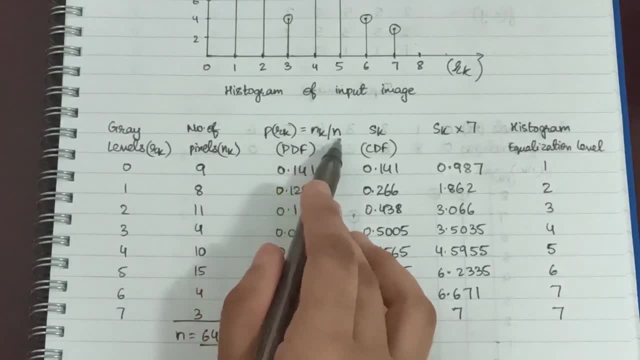 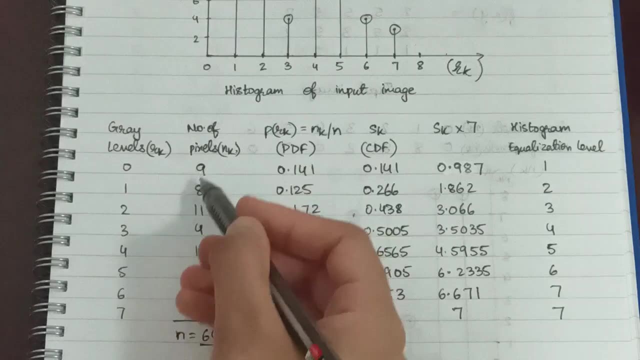 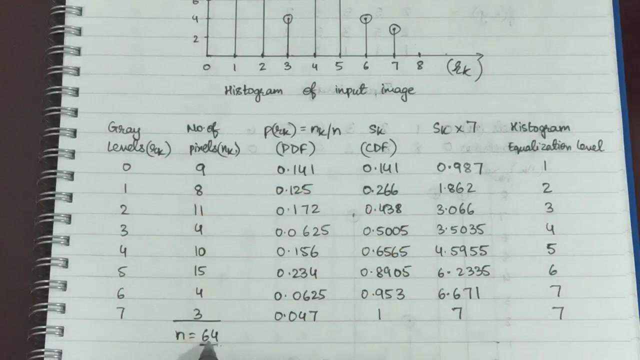 p of rk is equal to nk by n. nk is these values and n is the total number of pixels. So when we take the sum of each of these values, we get it as 64.. Now what we are doing here is we are taking 9 by 64, which is coming out to be 0.141.. We are taking 8 by 64. 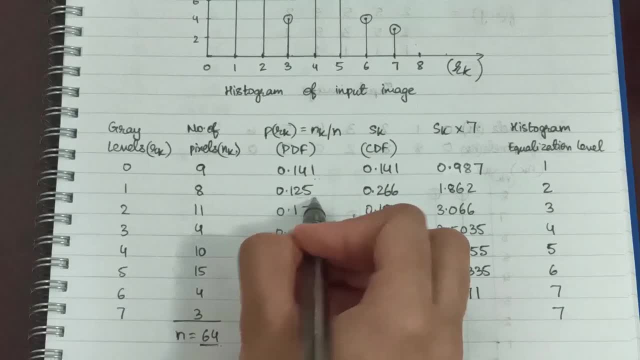 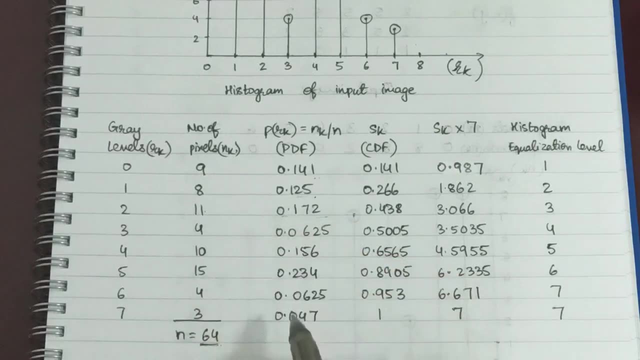 which is coming out to be 0.125.. Similarly here, 11 by 64- this is the value, 4 by 64- this is the value. So we are just dividing these values by 64 and writing down the answer here. Next comes cdf, or cumulative distribution function. So here this we are writing, representing: 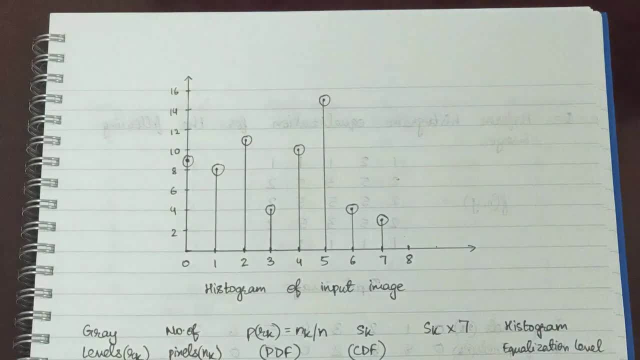 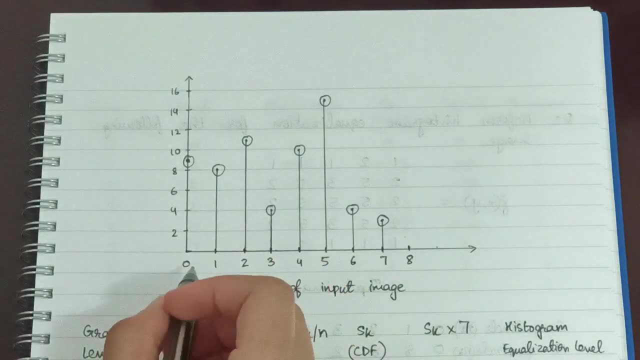 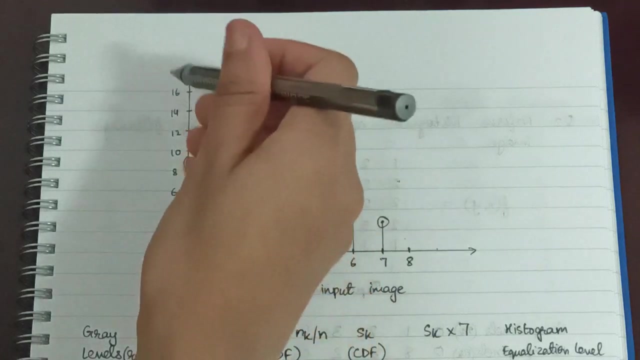 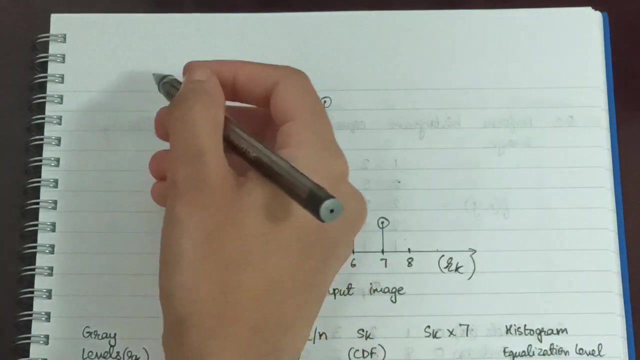 now, based on the above table, we can draw this histogram of input image here. okay, where all of these 0, 1, 2, 3, all of these represent the gray levels and these represent the number of pixels. so the x axis represents the gray level and the y axis represents the 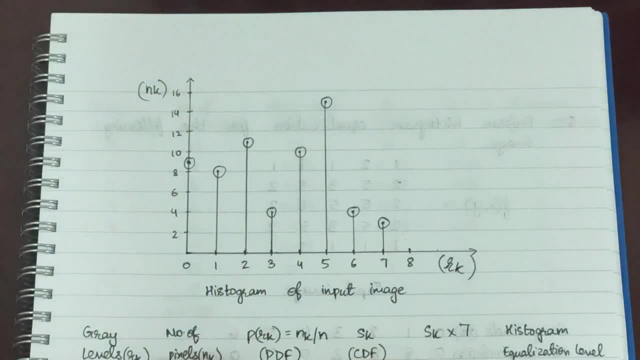 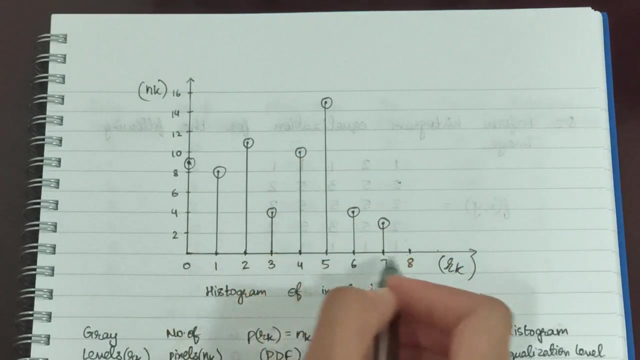 number of pixels. so you can see, for 0 we have the value 9- okay, which was given in the previous table- and similarly for 1 we have the value 8, for 2 it is 11, for 3 it is 4 and so on. so we have marked. 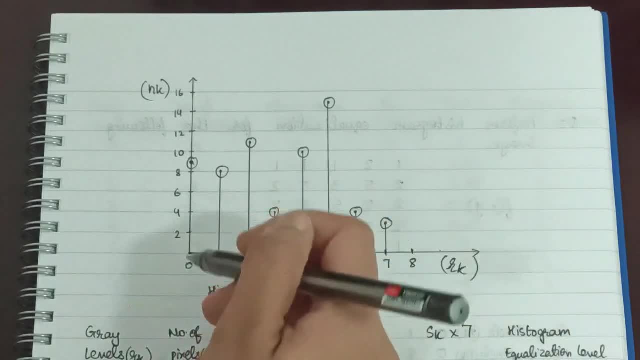 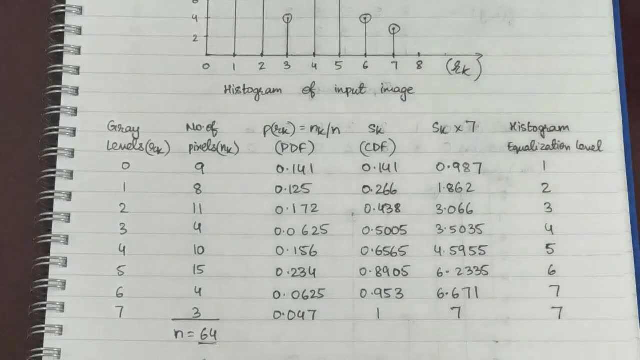 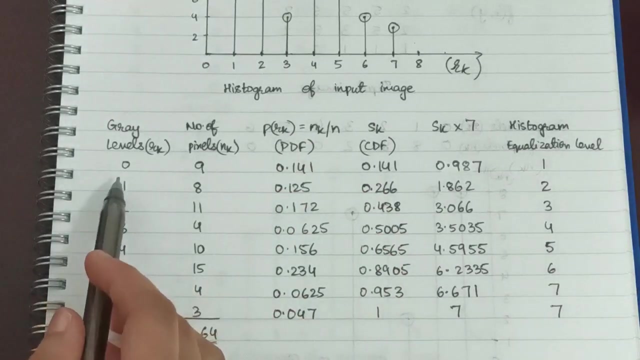 each of these gray levels and their number of pixels in this histogram here. next we are forming the table here: the gray level values and the number of pixels. we have just written it down from the question. okay, each of these values, we have written it down and now we 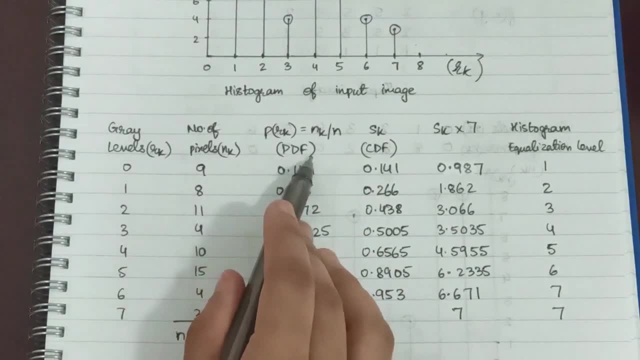 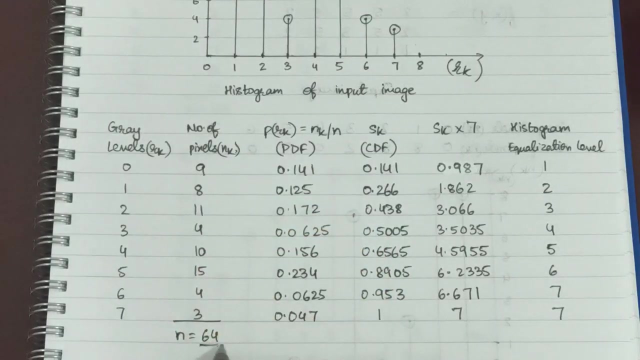 calculate the probability distribution function. so this is: p of rk is equal to nk by n. nk is these values and n is the total number of pixels. so when we take the sum of each of these values, we get it as 64. now what we are doing here is we are taking 9 by 64, which is coming out to be: 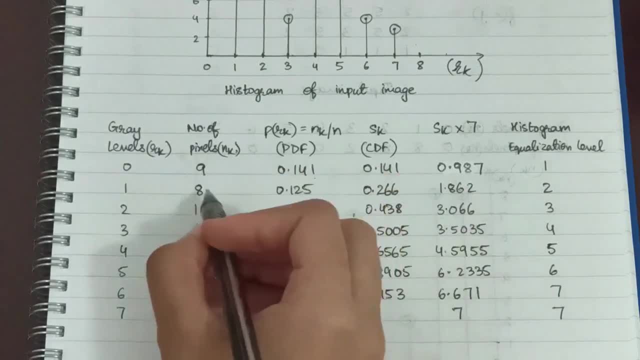 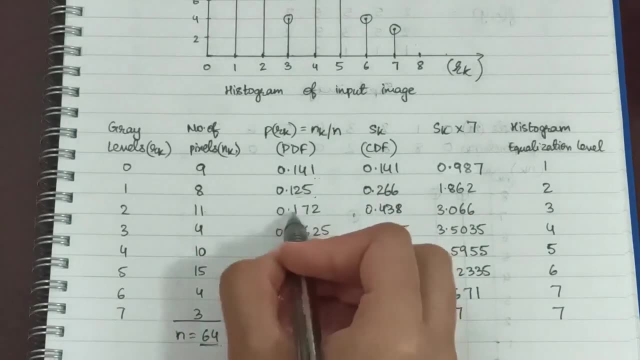 0.141. we are taking 8 by 64, which is coming out to be 0.125. similarly here, 11 by 64- this is the value. 4 by 64- this is the value. so we are just dividing these values and we are getting the total number of pixels. so we are taking 8 by 64, which is 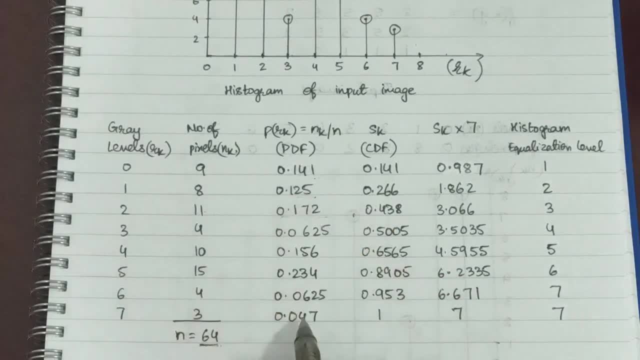 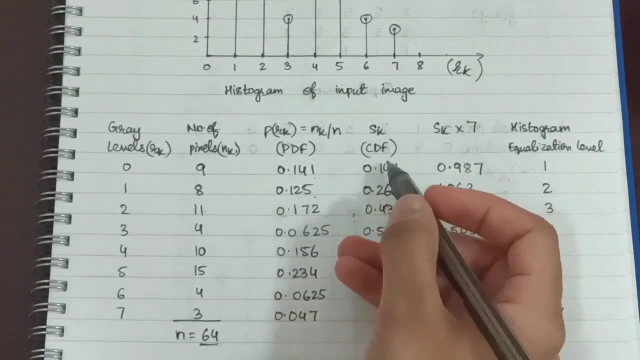 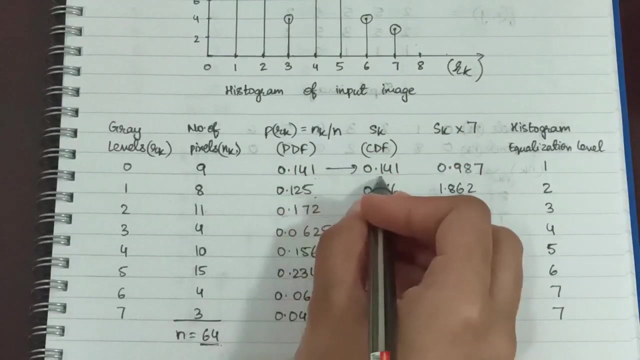 these values by 64 and writing down the answer here. next comes cdf or cumulative distribution function. so here this we are writing, representing as sk, and what we are doing. see directly: this value comes here. okay, but for calculating the next value we just add this value and this value. 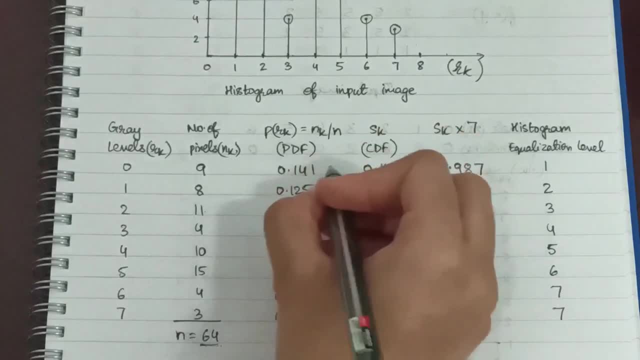 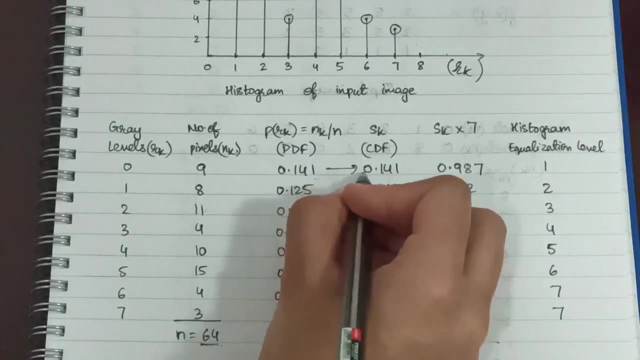 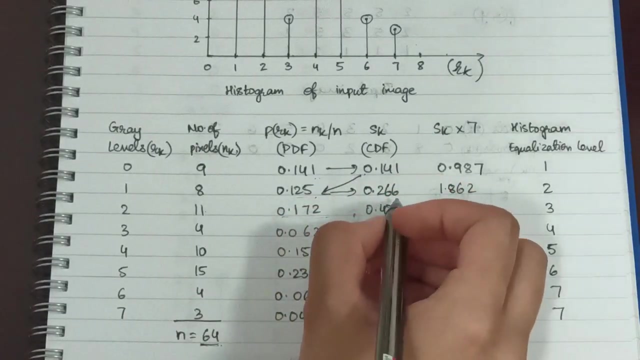 as sk and what we are doing. see directly. this value comes here. okay, But for calculating the next value, we just add this value and this value and the sum of this we write it down here, which is coming out to be 0.266.. Now, this 0.266 we are adding with this value. 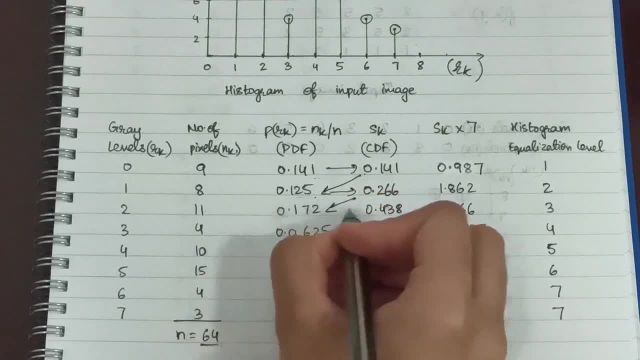 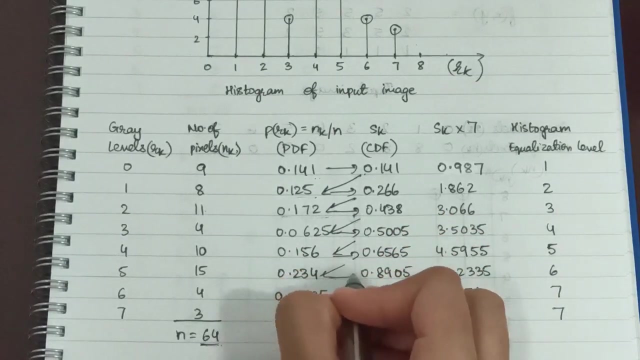 0.172 and the sum we are writing it down here, which is coming out to be 0.438.. Similarly, we are taking the sum of these two and writing it down here: Sum of this and this, writing it down here. So, like that, we keep going on and on And here we are getting. 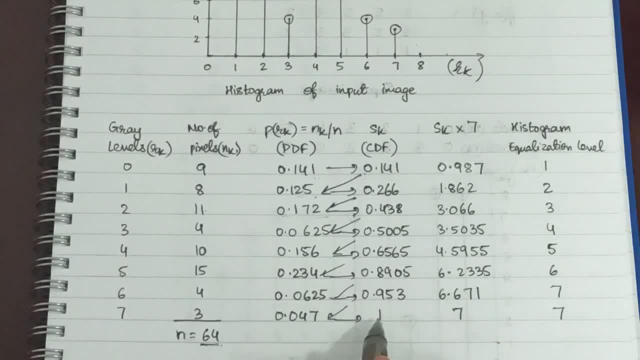 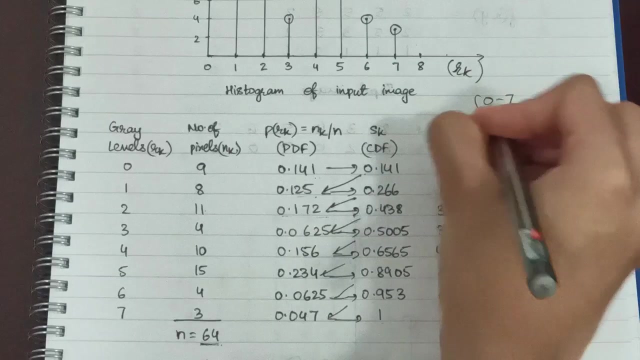 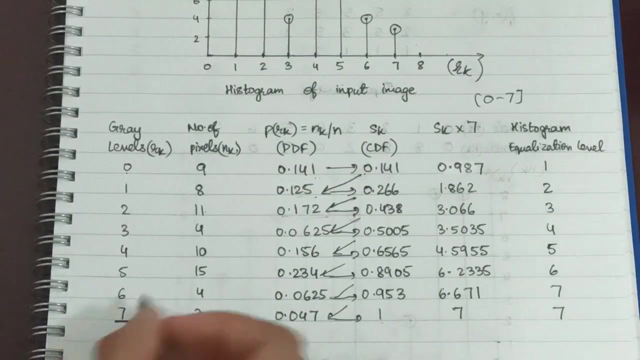 1 as the answer. Next, column sk into 7.. So we are just taking these column values and multiplying it by 7. why 7? because, if you see, our interval is from 0 to 7. okay, the first value, 0, last value, 7. so, since this is our last interval value, that's where. that's why we are multiplying. 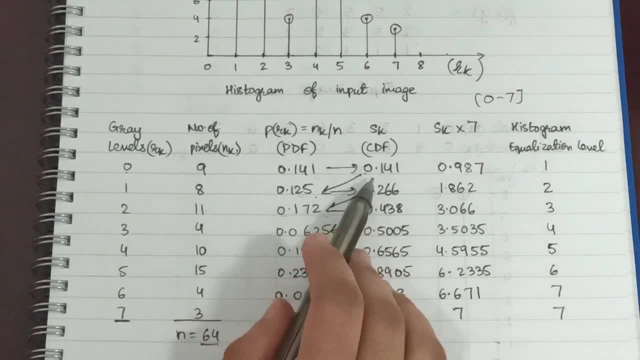 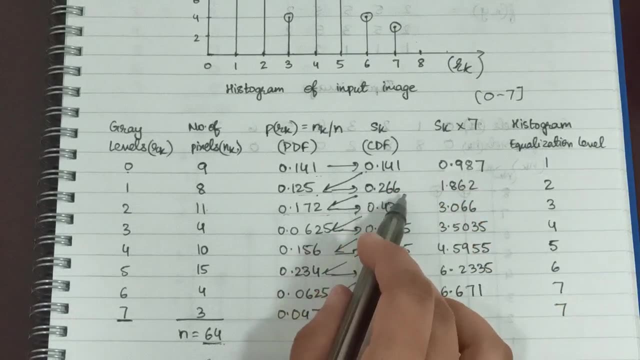 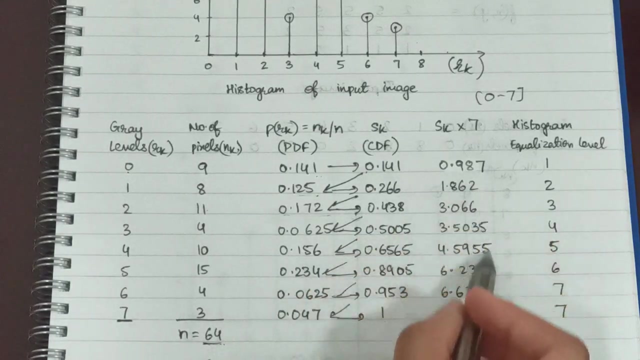 it by 7: 0.141 into 7, it is coming out to be 0.987, 0.266 into 7, which is coming out to be 1.862. so, similarly, each of these values, we are multiplying by 7 and getting these values. 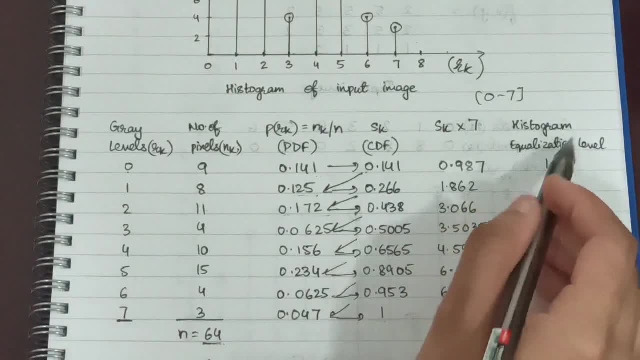 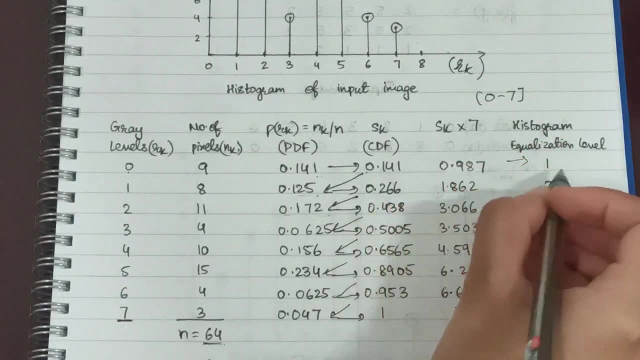 next column is histogram equalization level. so here we're just rounding off these values. okay, so just the round off of this is 1. rounding off this value, it's coming out to be 2. this value is coming out to be 3, 3.5. we have taken 4, 4.5. we have taken 5. so if it is 0.5. 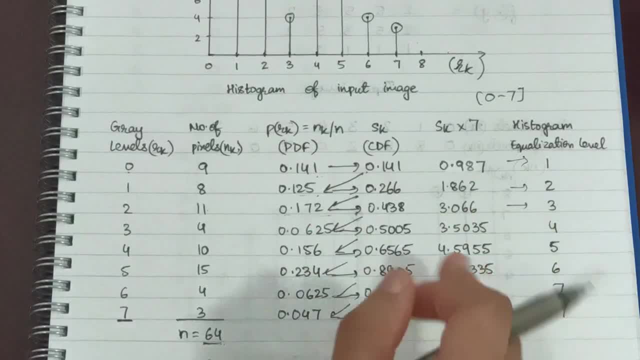 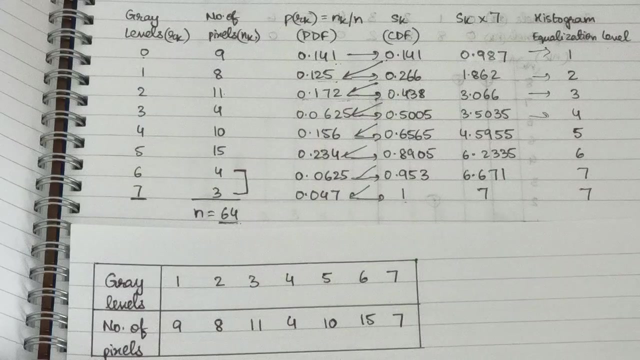 then it is the next value, right? if it is less than 0.5, then we are taking the previous value, see normal round off in decimal convention. so we have just rounded, rounded off all of these values and we have got these values. now what we did is these histogram equalization level values. we have just written it down. 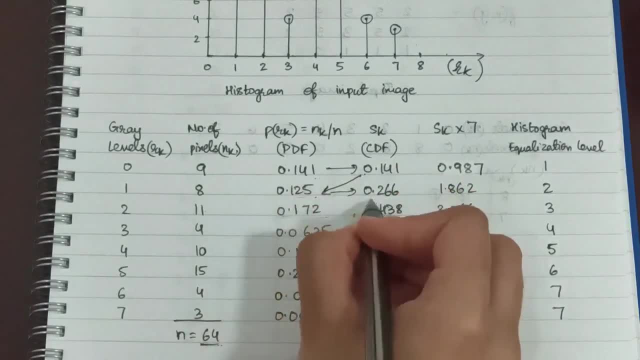 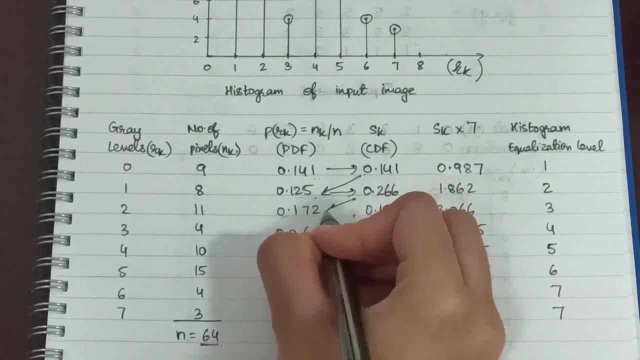 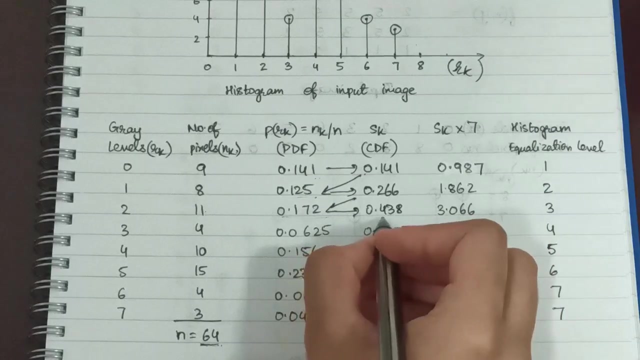 and the sum of this- we write it down here- which is coming out to be 0.266. now, this 0.266, we are adding, with this value, 0.172, and the sum we are writing it down here, which is coming out to be 0.438. similarly, we are taking the sum of these two. 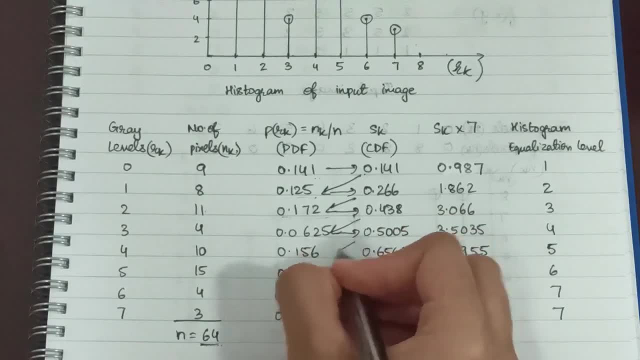 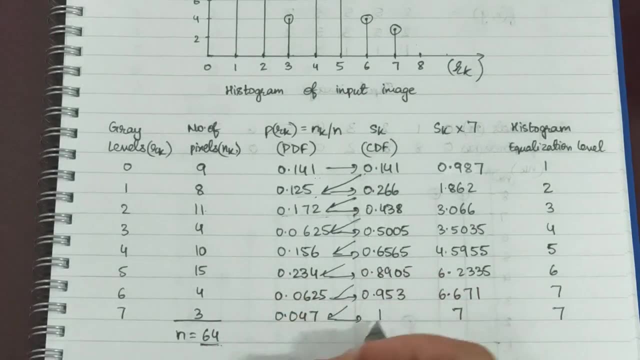 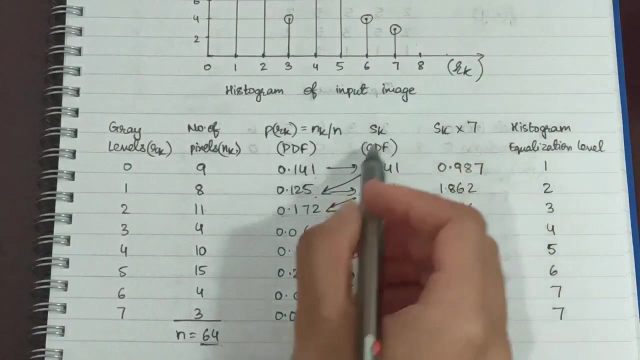 and writing it down here, some of this and this writing it down here. so like that, we keep going on and on and here we are getting one as the answer. next, column sk into 7. so we're just taking these column values and multiplying it by 7. why 7? because, if you see, 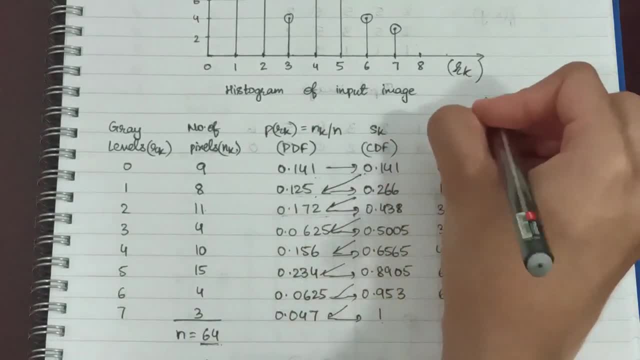 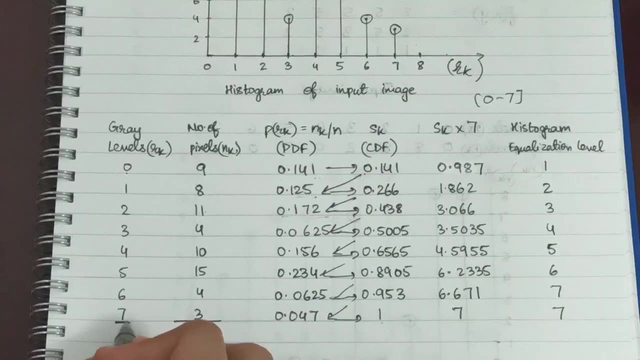 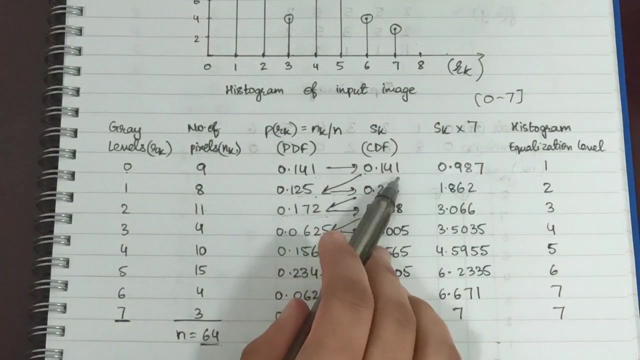 our interval is from 0 to 7. okay, the first value, 0, last value, 7. so since this is our last interval value, that's where that's why we are multiplying it by 7: 0.141 into 7, it is coming out to be 0.987. 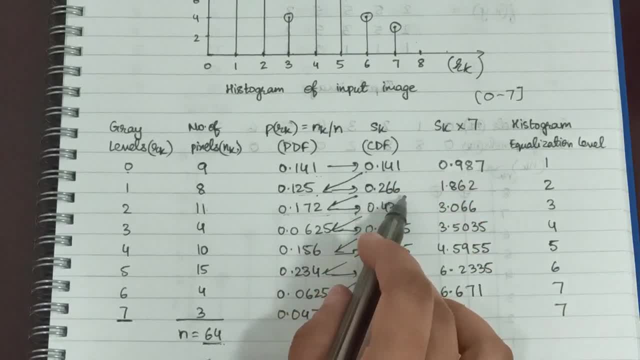 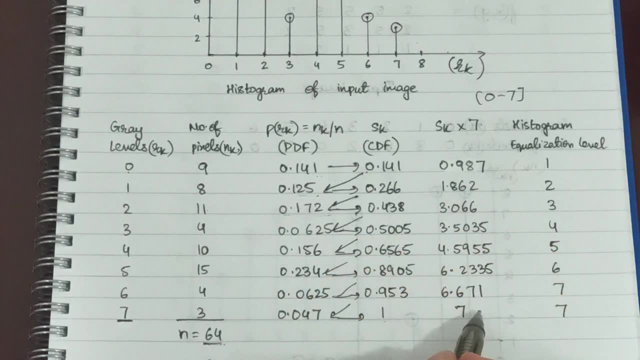 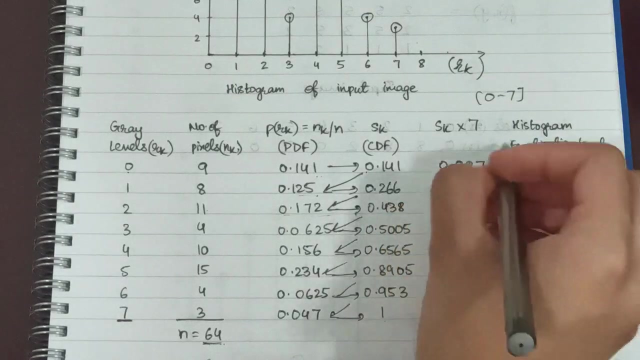 0.266 into 7, which is coming out to be 1.862. so, similarly, each of these values, we are multiplying by 7 and getting these values. next column is histogram equalization level. so here we're just rounding off these values. okay, so just the round off of this is 1 rounding off this value. it's. 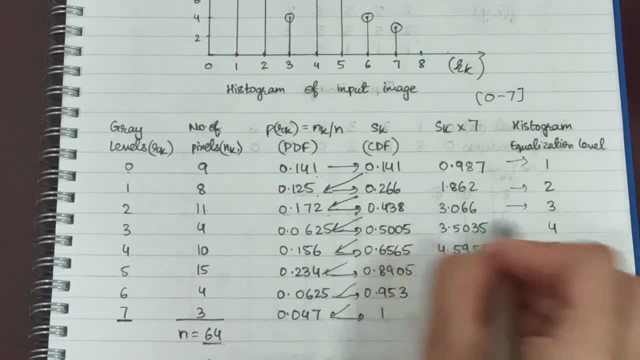 coming out to be 2. this value is coming out to be 3- 3.5. we have taken 4- 4.5. we have taken 5- 4.5. we have taken 4- 4.5. we have taken 5. 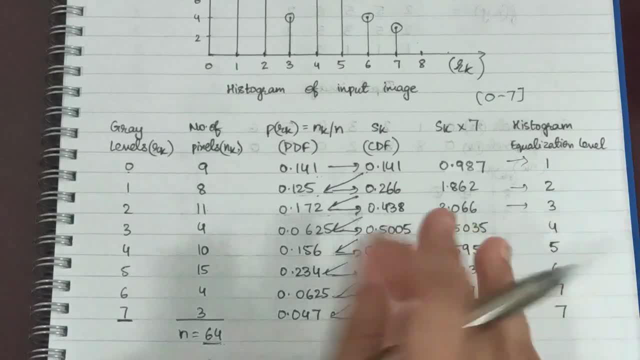 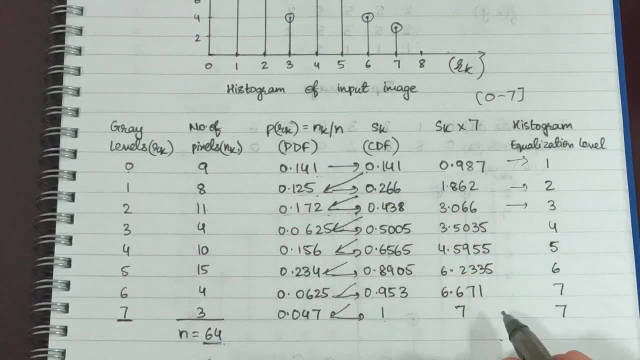 so if it is 0.5, then it is the next value, right? if it is less than 0.5, then we are taking the previous value, see normal round off in decimal convention. so we have just rounded, rounded off all of these values and we have got these values. now what we did is these histogram equalization. 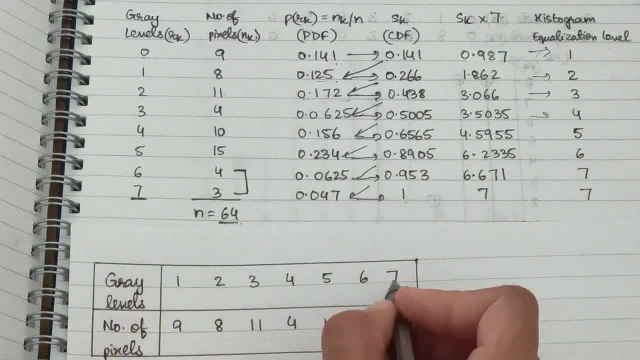 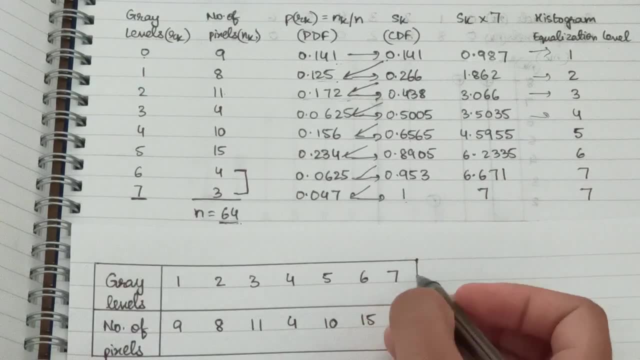 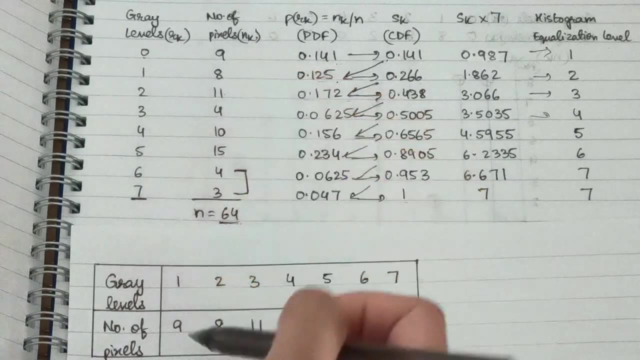 level values. we have just written it down as our new gray level values, okay as it is. and for here, 7 has come twice, so we just wrote it once. and for the number of pixels, we have taken down this column: okay, these values. you can see here these corresponding values, and what we have done is that. 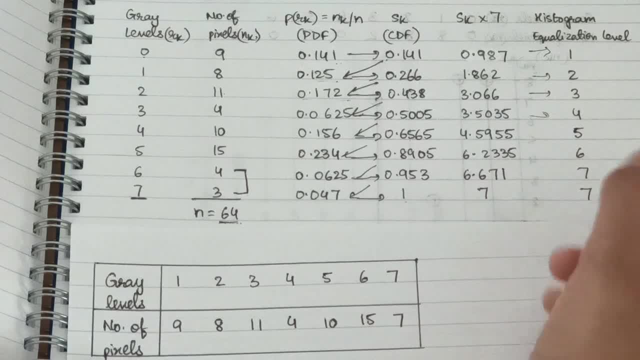 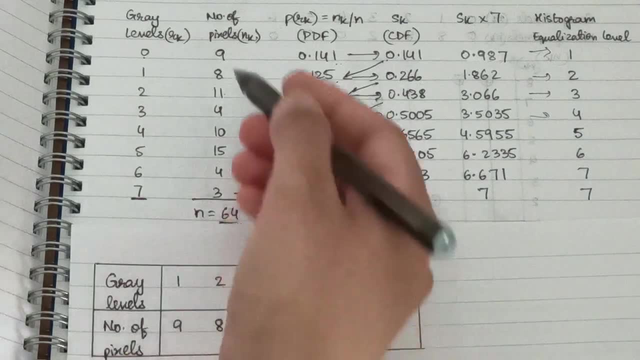 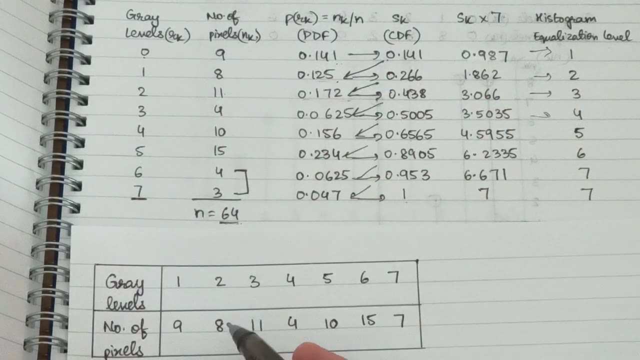 as our new gray level values. okay, as it is, and for here, 7 has come twice, so we just wrote it once. and for the number of pixels, we have taken down this column. okay, these values. you can see here these corresponding values, and what we have done is that for 7, which has come. 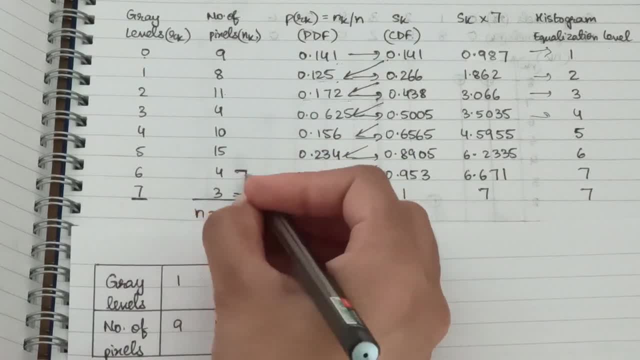 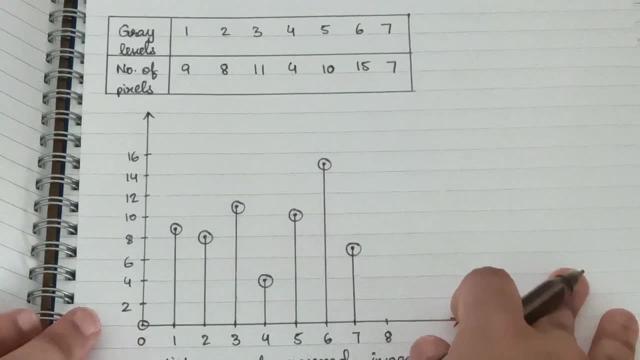 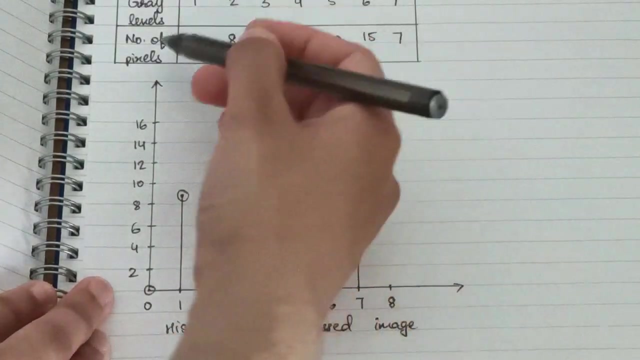 twice. we have taken the sum of 4 and 3, okay, these two values, which has come out to be 7, and after this we do the histogram here. so this is the histogram of processed image and this is based on these values. What we did is: 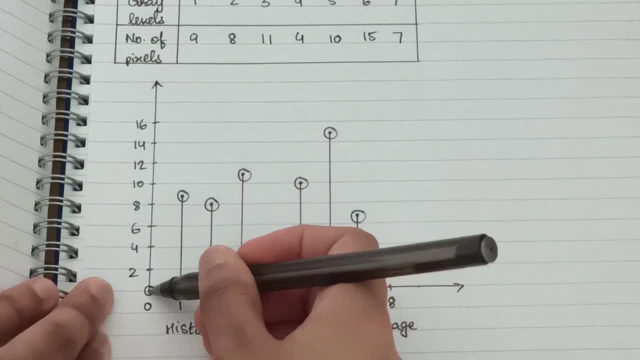 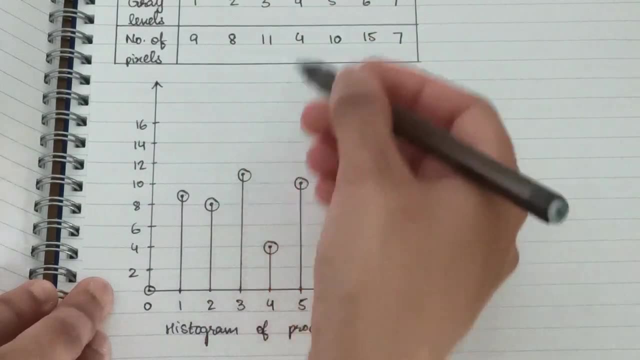 okay, you can see. for 0 we don't have any value, so we have just marked at 0. for 1 it has the value 9, so we marked it at 9. for 2 it is 8. for 3 it is 11. so 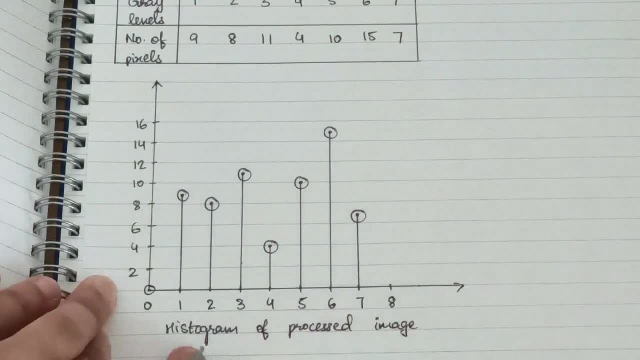 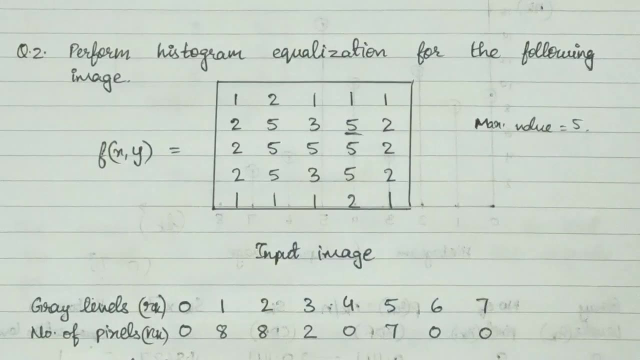 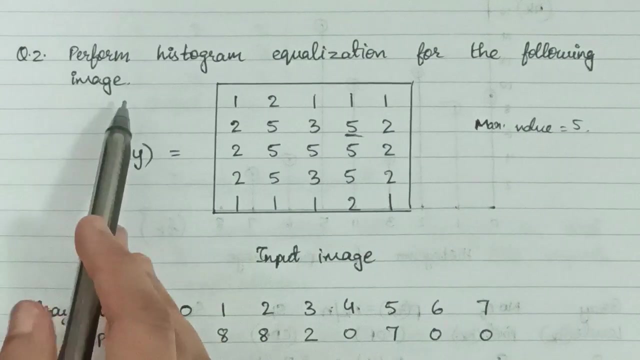 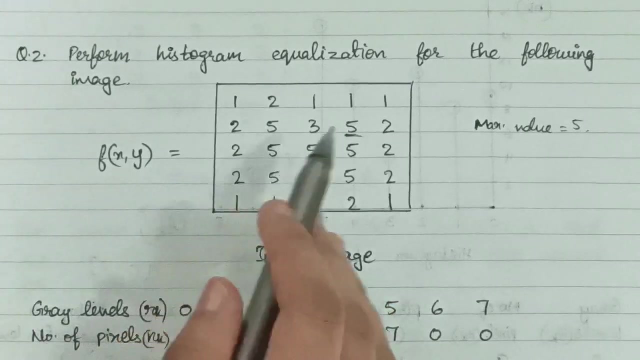 accordingly. we have marked all the values and this is the histogram of the processed image. now let's look at one more example here. perform histogram equalization for the following image: we have a direct image here and we need to do the histogram equalization, but we don't have the number of pixels here directly, right? so? 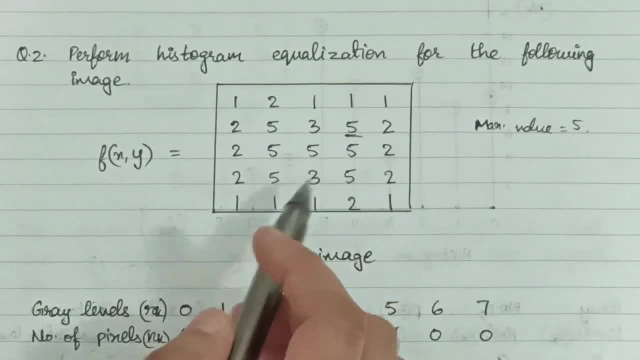 how will we calculate the table? what we do is we take the maximum pixel value here, okay, which means that the maximum pixel value here we have 1, 2, 3 & 5, right, so 5 is the maximum value. now we will try to represent this maximum value. flower. 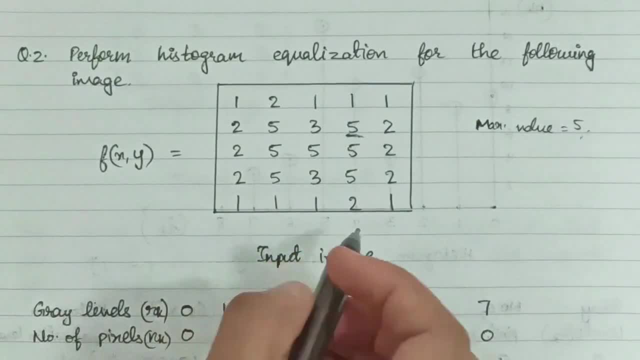 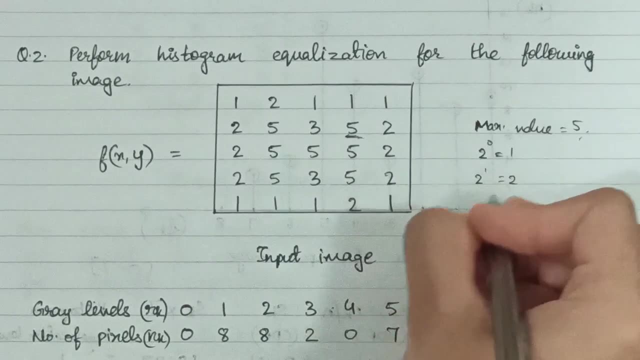 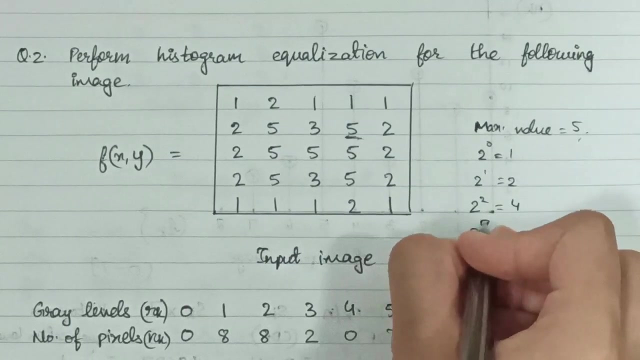 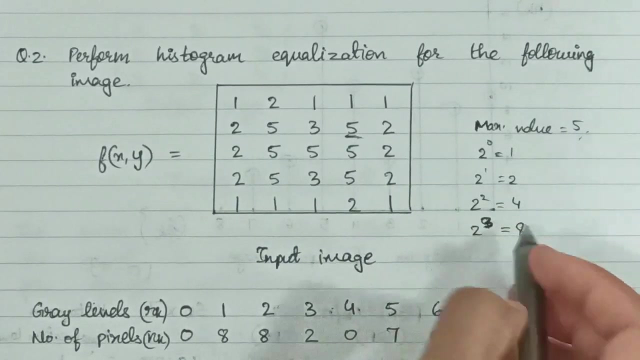 terms of powers of 2. okay, so if we take 2 of 0, it comes out to be 1. 2 of 1 it comes to 2. square is 4. 2 raised to 4 is sorry. 2 raised to 3 is 8. right now, 5 is less than 8, so that's why we choose this. 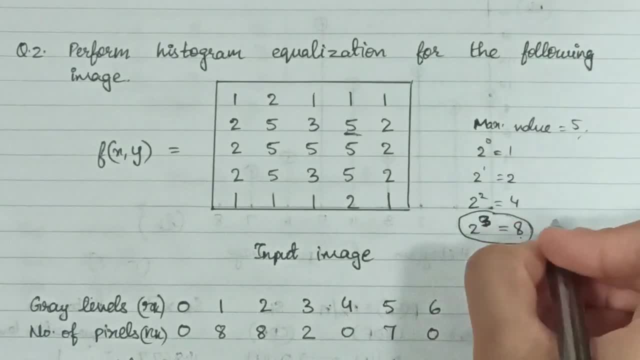 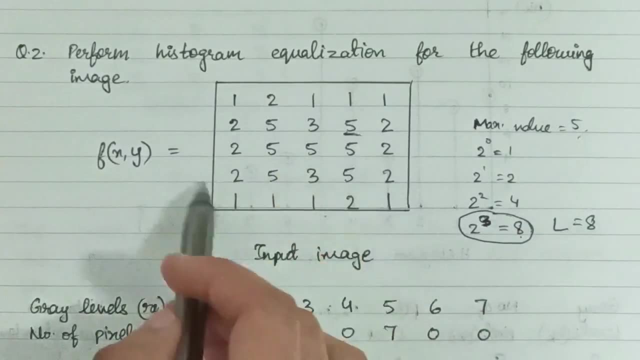 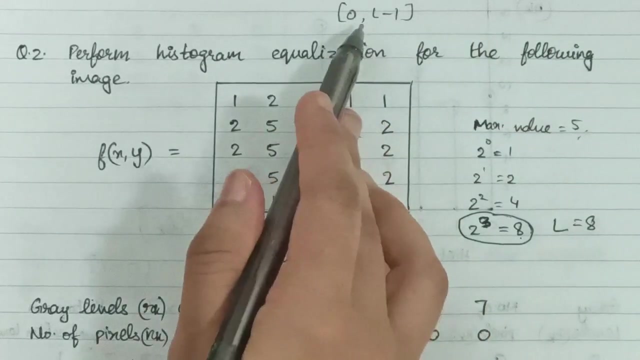 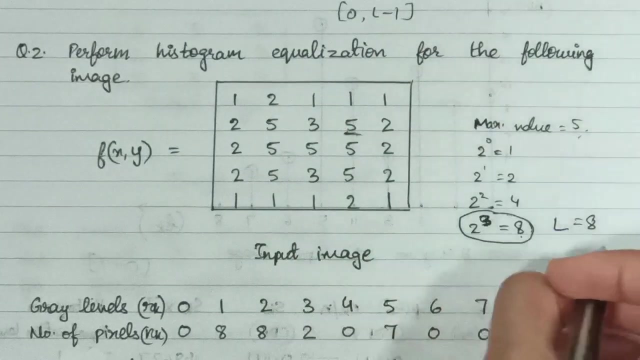 1. now we choose l is equal to 8. remember l see, we represent these pixels in the interval 0 to l minus 1, right? this we had studied in our previous lectures. so this 0 to l minus 1 is our interval. so if l is 8, then we have l minus 1 equal to 7. so what we'll do is our gray levels. 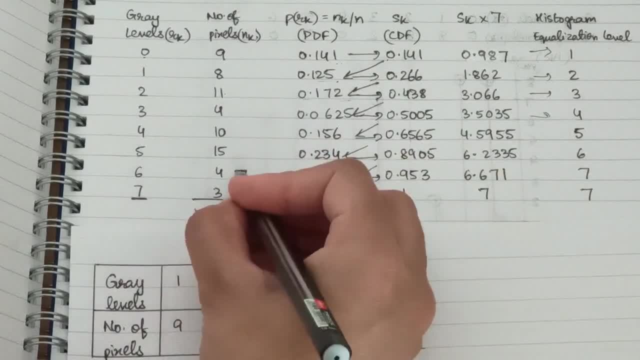 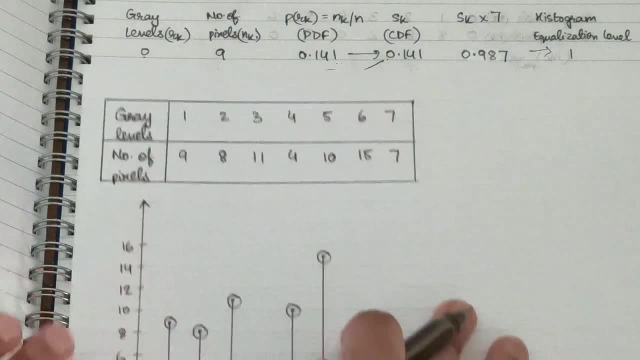 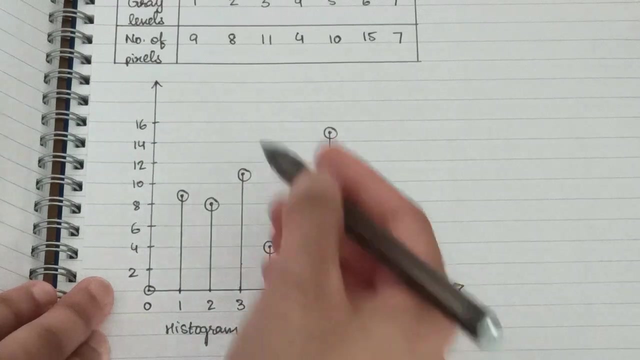 for 7, which has come twice, we have taken the sum of 4 and 3, okay, these two values, which has come out to be 7, and after this we do the histogram here. so this is the histogram of processed image and we this is based on these values. okay, you can see. for 0, we don't have any value, so we. 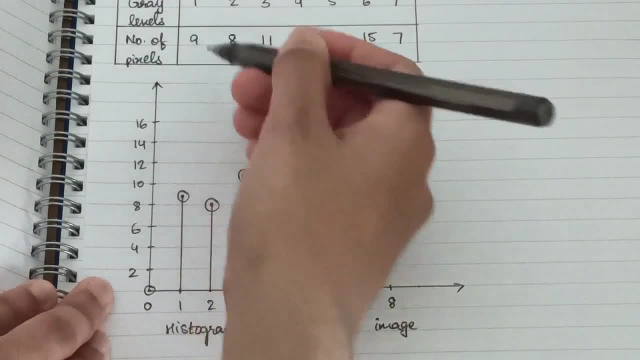 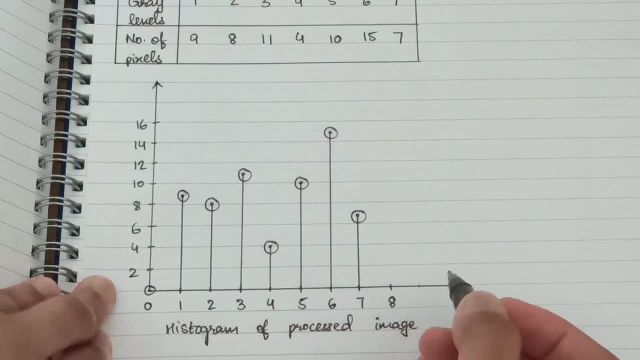 have just marked it as 0. for 1 it has the value 9, so we marked it at 9. for 2 it is 8. for 3 it is 11, so accordingly we have marked all the values and this is the histogram of the processed image. 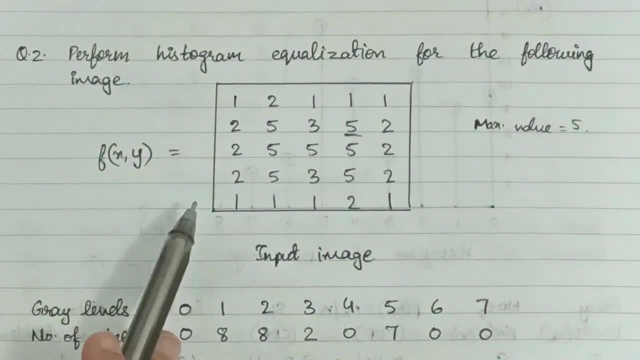 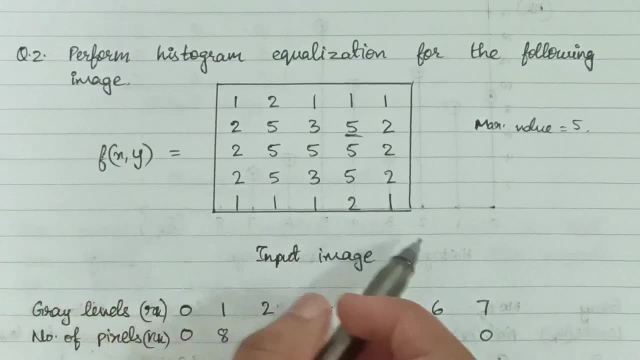 now let's look at one more example here. perform histogram equalization for the following image. we have a direct image here and we need to do the histogram equalization, but we don't have the number of pixels here directly, right? so how will we calculate the table? 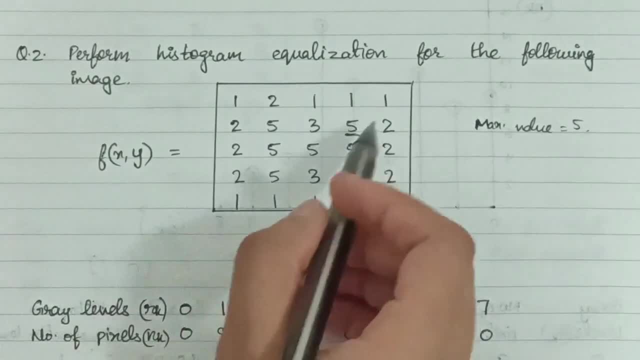 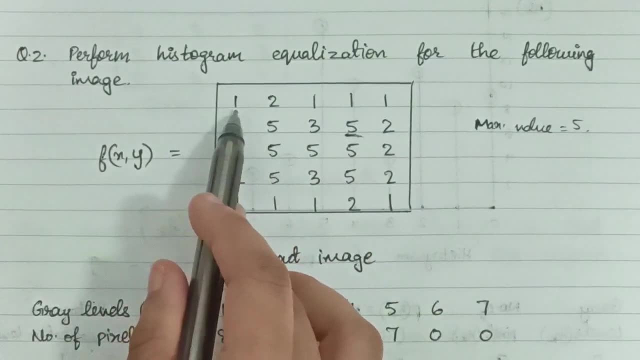 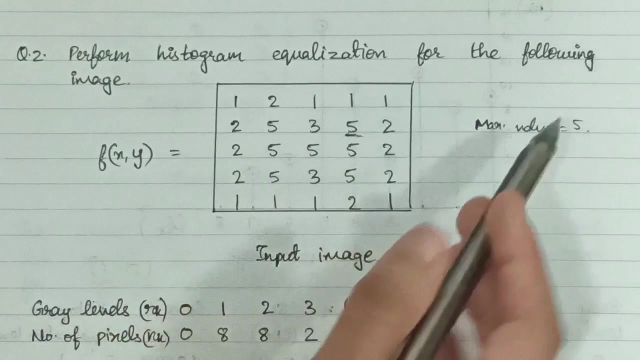 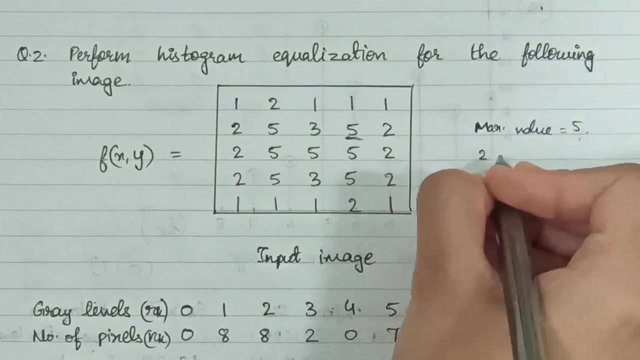 what we'll do is we take the maximum pixel value here, okay, which means that the maximum pixel value here we have 1, 2, 3 and 5, right, so 5 is the maximum value. now we'll try to represent this maximum value in terms of powers of 2. okay, so if we take 2 of 0, it comes out to be 1, 2 of 1 it comes to 2. square is 4. 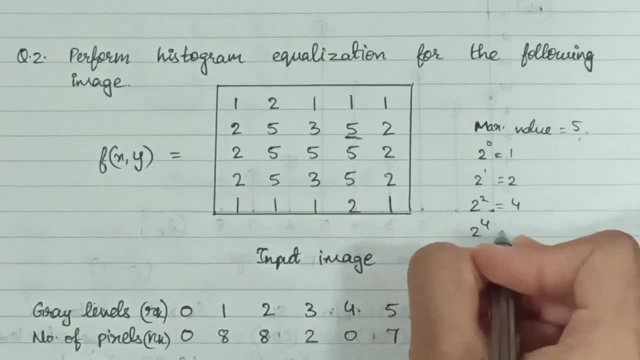 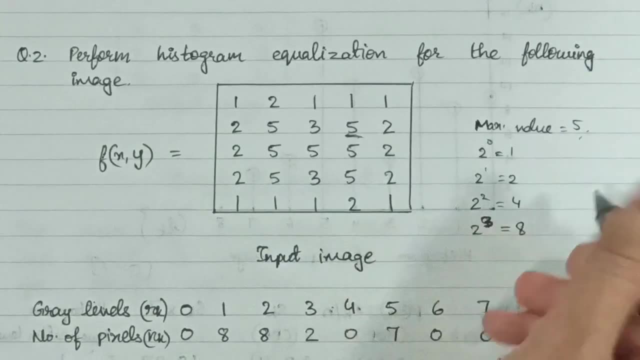 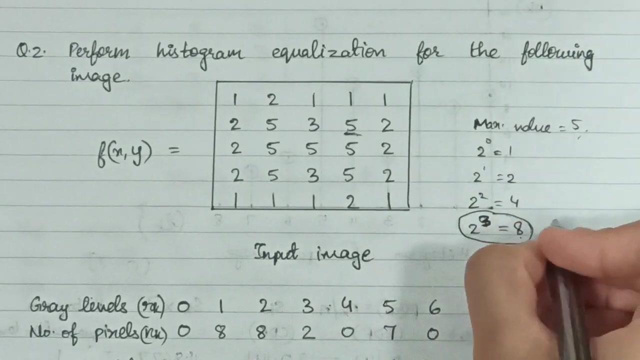 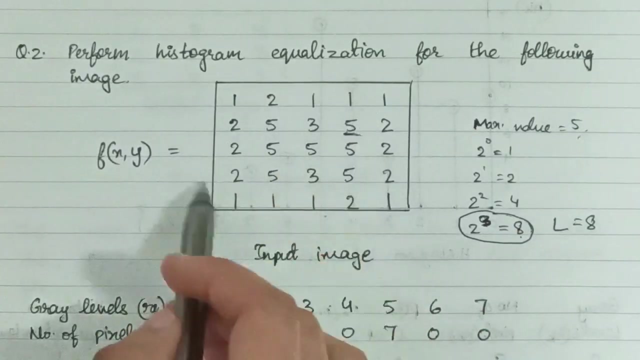 2 raised to 4 is sorry. 2 raised to 3 is 8. right now, 5 is less than 8, so that's why we choose this one. now we choose: l is equal to 8. remember l see. we represent these pixels in the interval 0 to l minus 1, right, this we had. 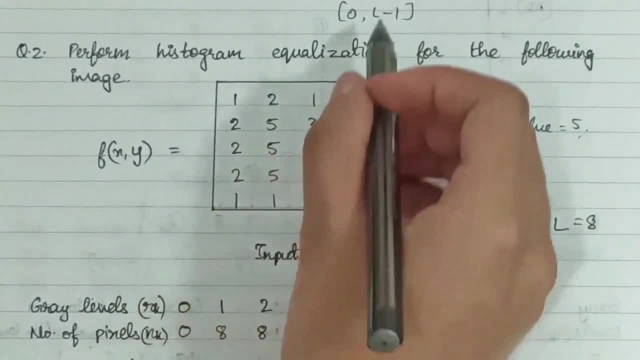 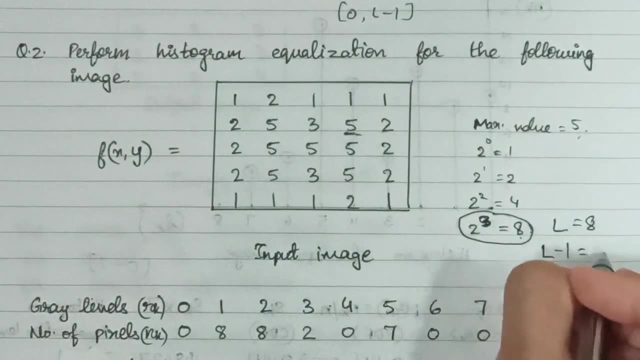 studied in our previous lectures. so this 0 to l minus 1 is our interval. so if l is 8, then we have l minus 1, equal to 7. so what we'll do is our gray levels will be from 0 to 7. okay, so what we'll do is: 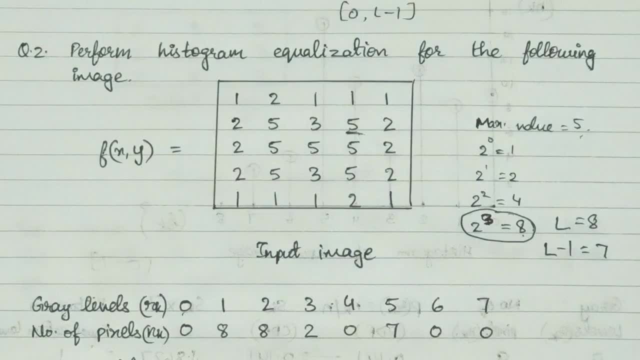 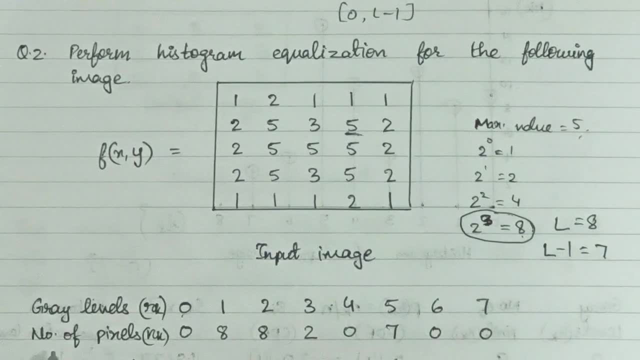 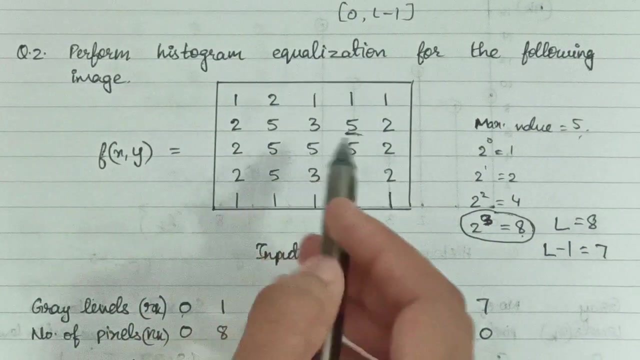 will be from 0 to 7, okay. so what we'll do is we just write down the gray levels from 0 to 7, okay, and the number of pixels. what we'll do is we'll check for the frequencies of each of these values, which means that 0 does not occur in this image. so we have the number of pixels: 0. 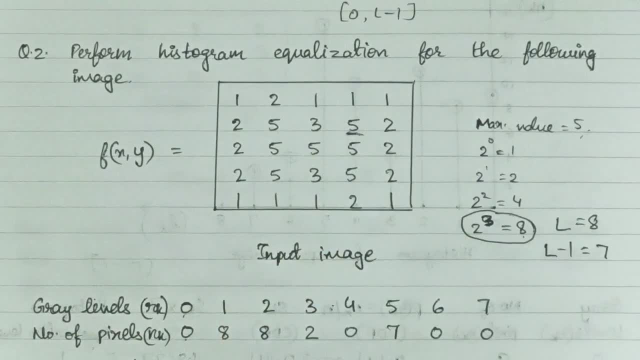 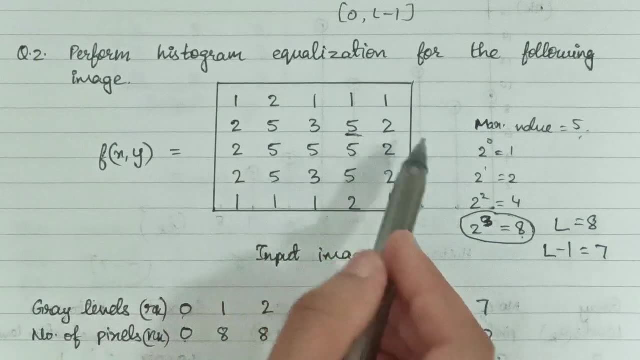 1 occurs 8 times in the image. 1, 2, 3, 4, 5, 6, 7, 8, so we have written 8. similarly, 2 occurs 8 times, so we have written 8 here. so, like that, we'll fill up this table. 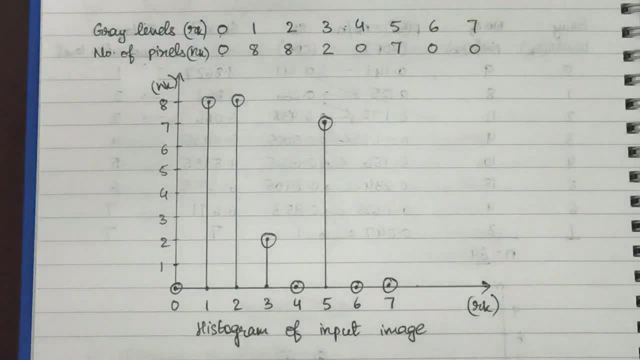 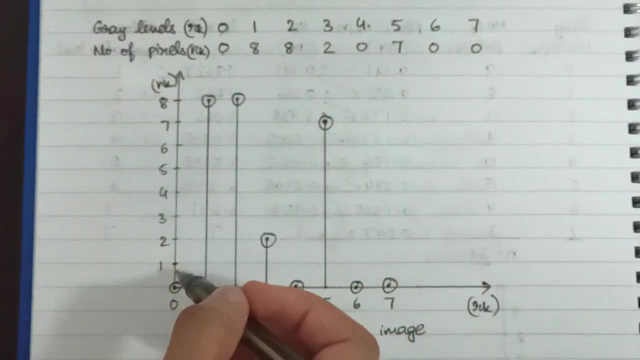 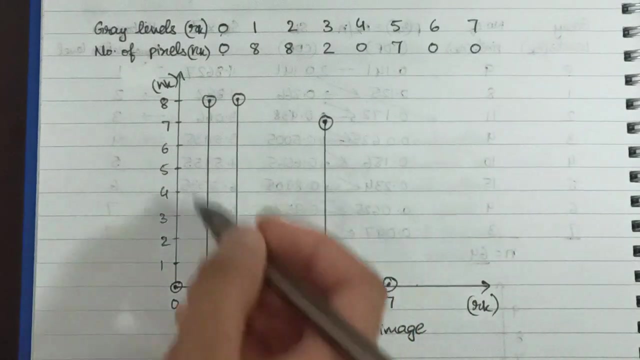 now, based on this table, we'll draw the histogram of the input image. for 0, the value is 0, right? so we just represent 0 here. for the gray level 1, the number of pixels is 8, so we have represented 8 here. for 2, also, it is 8, so we have marked 8 here. for 3, it is 2, so similarly for all of the values. 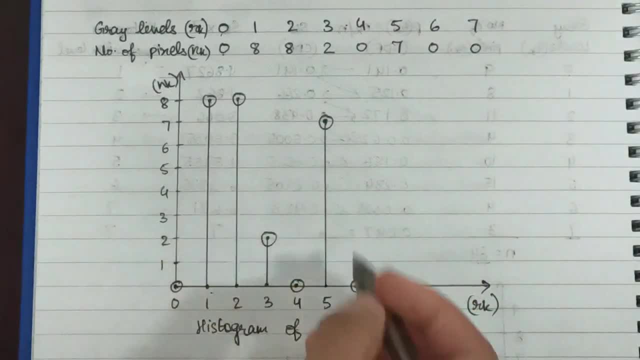 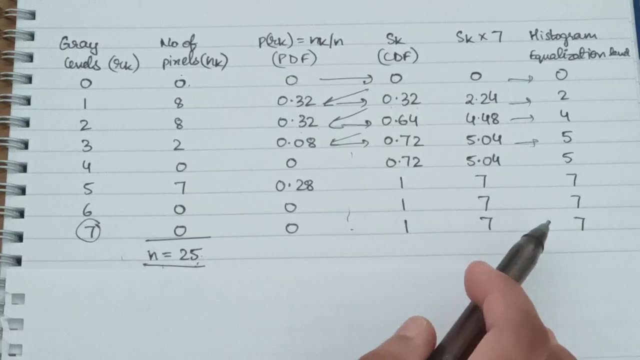 we'll draw the histogram values here now. we have drawn a table here. okay, similar as the previous problem. here we have written down the gray levels and the number of pixels. we calculated the total pixels, which is 25. then we calculated pdf, which is nothing but each of these values divided by 25. 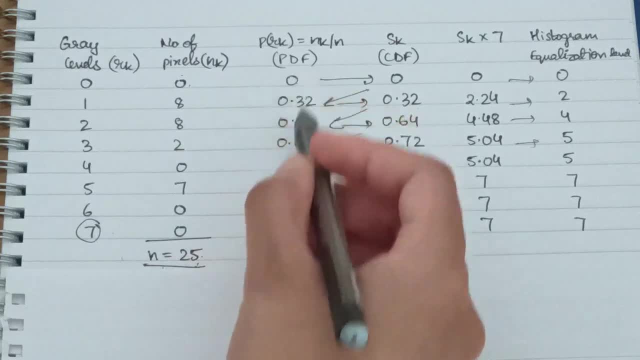 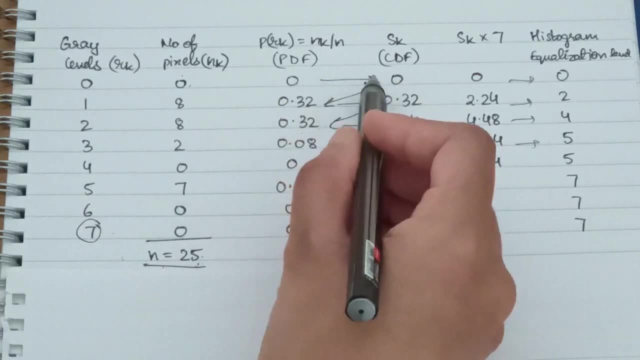 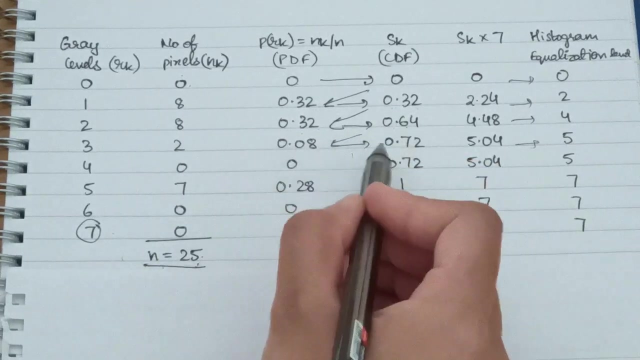 0 by 25, 8 by 25- we have just written down the values here. then we calculated cdf, which is nothing but 0, for this value which just comes directly, and then 0 plus 0.32, which comes here, 0.32 plus 0.32, which comes here, and so on. so we got this column and then we multiply this column. 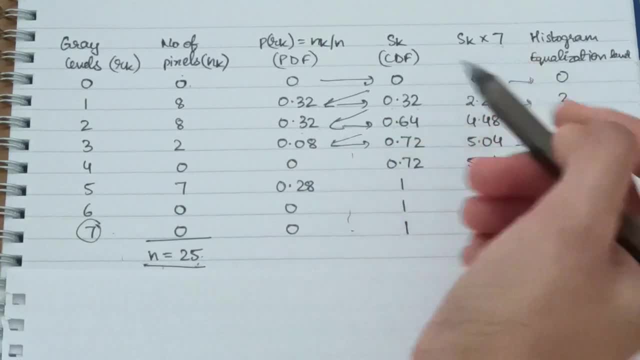 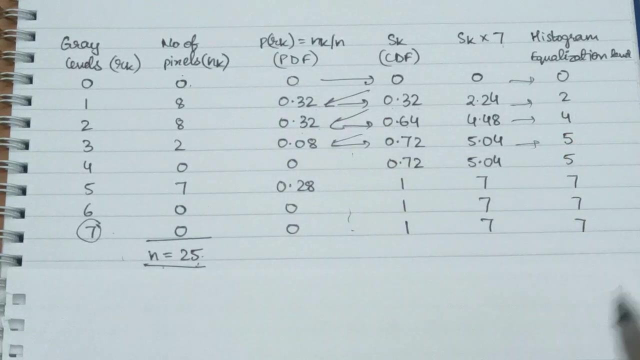 by 7. okay, why 7? because our interval was from 0 to 7. so after that, once we calculated these values, then we just rounded them off and we got histogram equalization levels, which is this column. so once we were done with that, then we. but then what we did is: 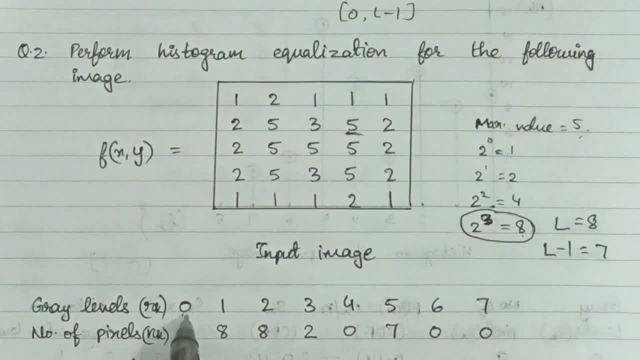 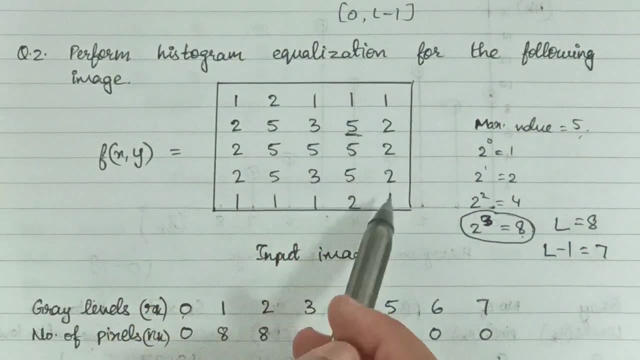 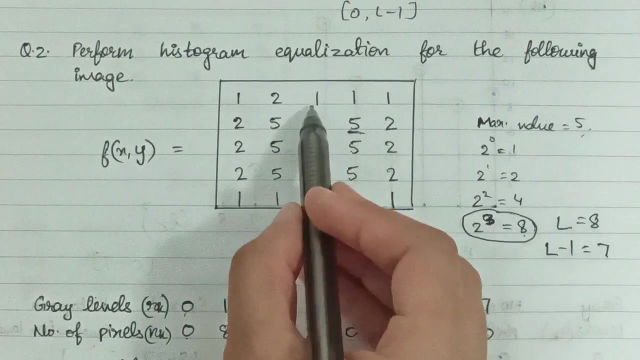 write down the gray levels from 0 to 7, okay, and the number of pixels. what we'll do is we'll check for the frequencies of each of these values, which means that 0 does not occur in this image, so we have the number of pixels: 0. 1 occurs 8 times in the image: 1, 2, 3, 4, 5, 6, 7, 8. so we have written 8. 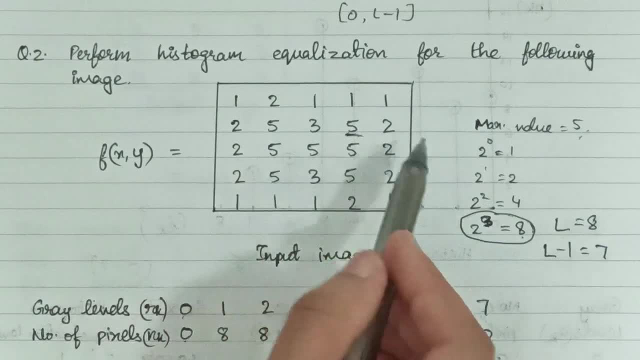 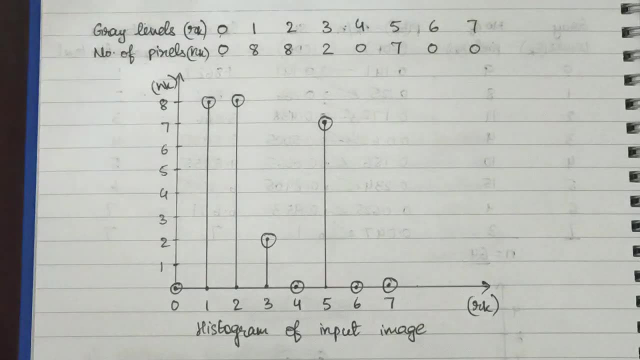 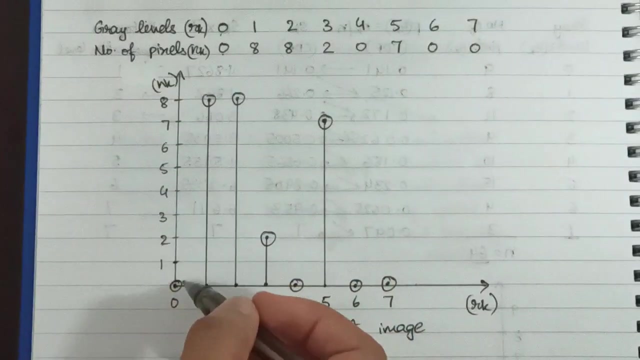 similarly, 2 occurs 8 times, so we have written 8 here. so, like that, we'll fill up this table now. based on this table, we'll draw the histogram of the input image. for 0, the value is 0, right, so we just represent 0 here. for the gray level 1, the number of pixels is 8, so we have represented. 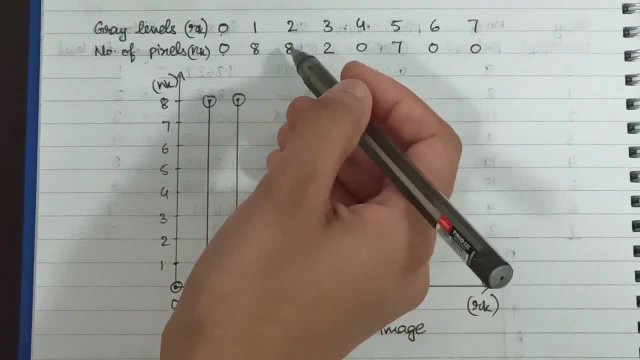 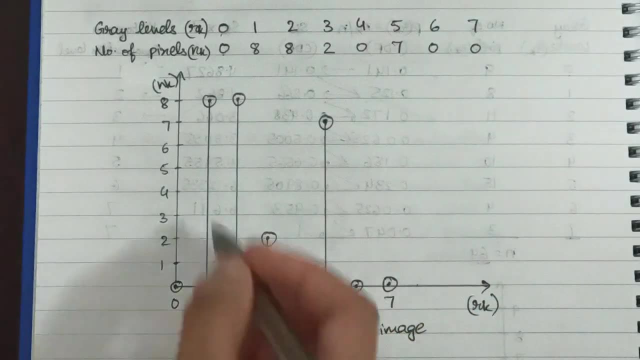 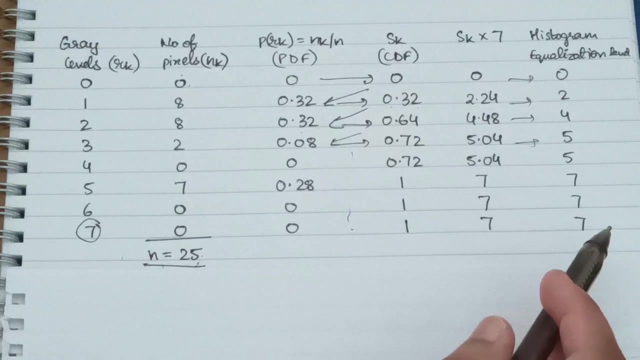 8. here for 2 also, it is 8. so we have marked 8. here for 3 it is 2. so similarly for all of the values. we'll draw the histogram values here. now we have drawn a table here. okay, similar as the previous problem. here we have written down the. 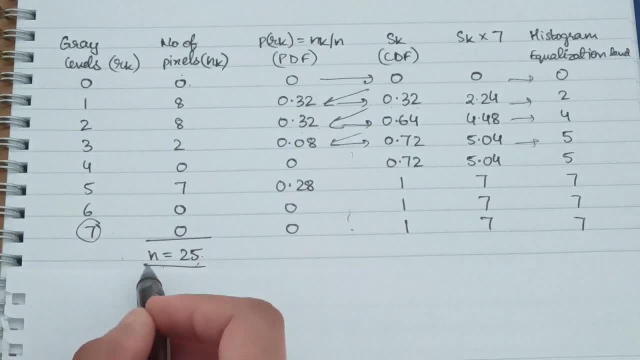 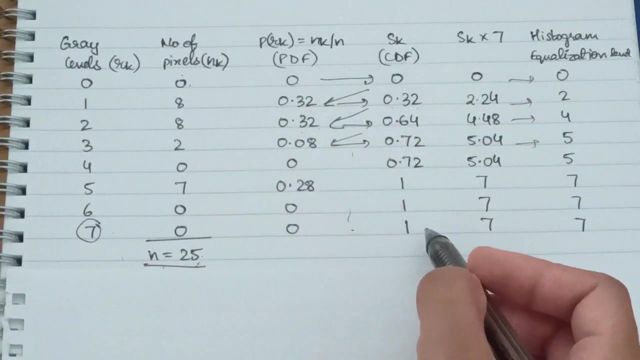 gray levels and the number of pixels. we calculated the total pixels, which is 25. then we calculated pdf, which is nothing but each of these values divided by 25, 0 by 25, 8 by 25. we've just written down the values here. then we calculated cdf, which is nothing but 0 for this value which just comes. 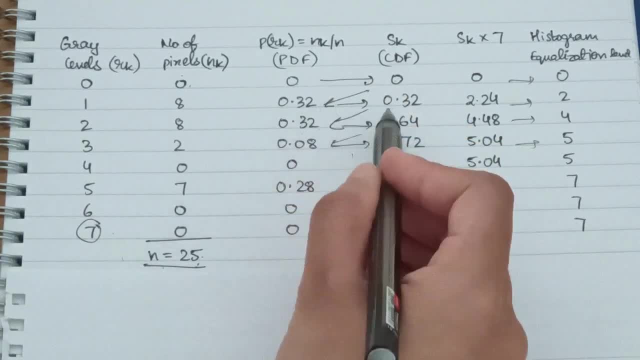 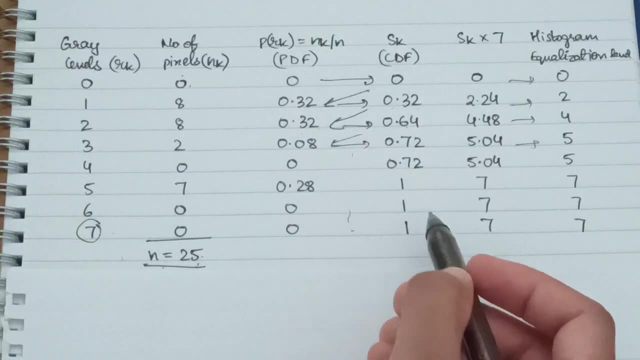 directly, and then 0 plus 0.32, which comes here, 0.32 plus 0.32, which comes here, 0.32 plus 0.32 which comes here, and so on. so we got this column and then we multiplied this column by 7. okay, why? 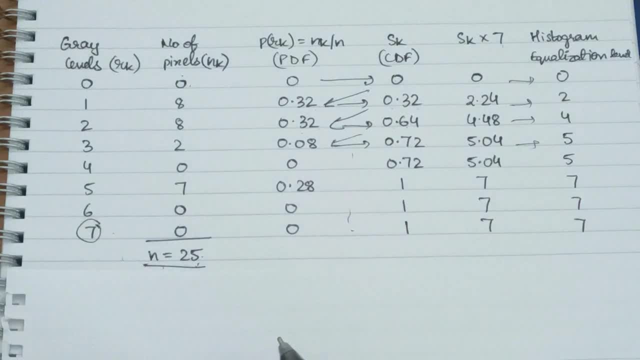 7, because our interval was from 0 to 7. so after that, once we calculated these values, then we just rounded them off and we got histogram equalization levels, which is this column. once we were done with that, then we. but then what we did is we drew this table: 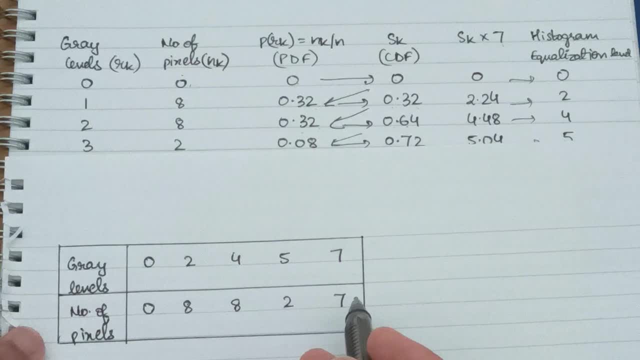 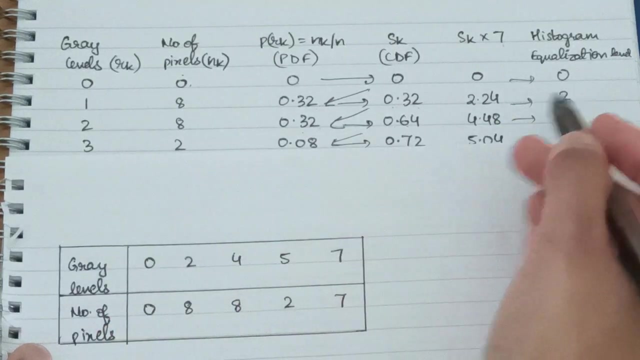 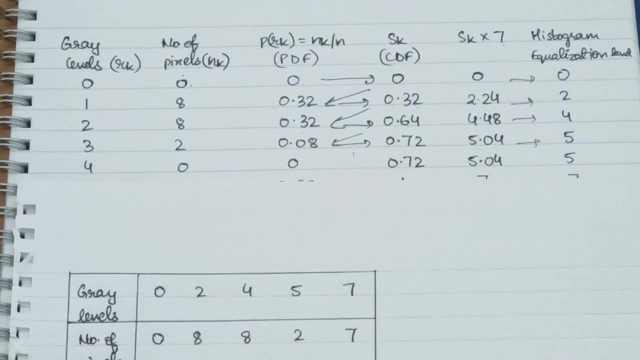 we drew this table. okay, here we have gray levels and number of pixels, the new gray levels. so this: these values are from the histogram: equalization levels: 0- we have just written it here. 2- we have written it here. 4- we have written it here, okay, 5. now what happened is that? 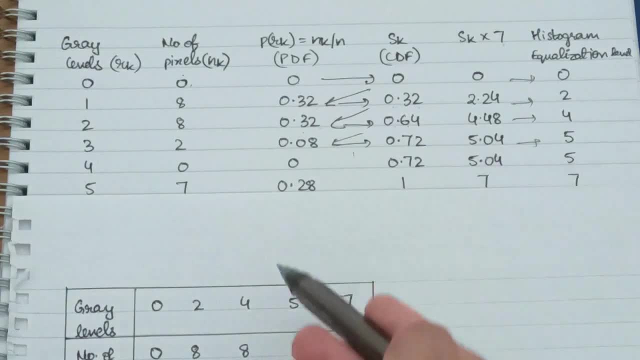 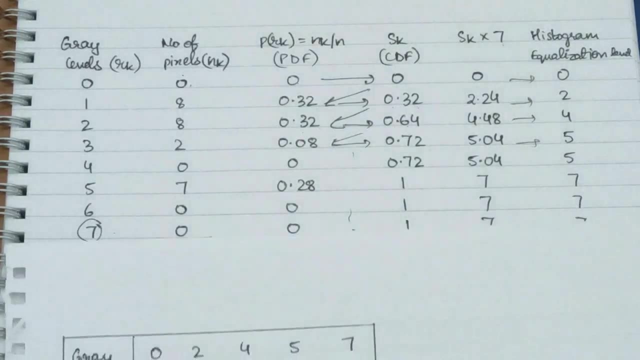 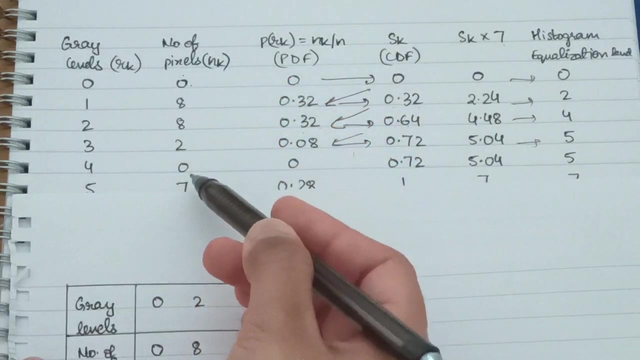 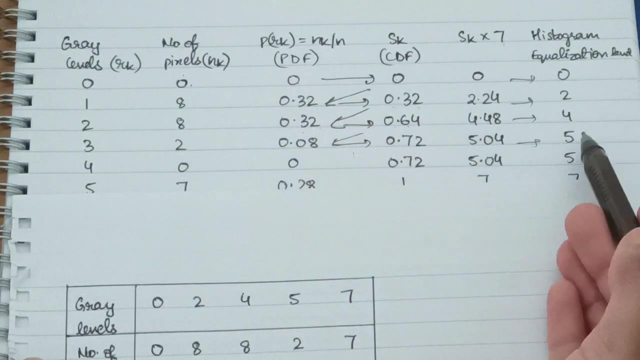 5 was twice. okay, over here, we just wrote it once. and similarly, 7 was thrice, if you see this. so we have that too. we have just written down once, and then we have written the corresponding number of pixels. for 0, it was 0. for 2, it was 8. for 4, it was 8 for 5, since 5 was 2 times. so we took the sum of these. 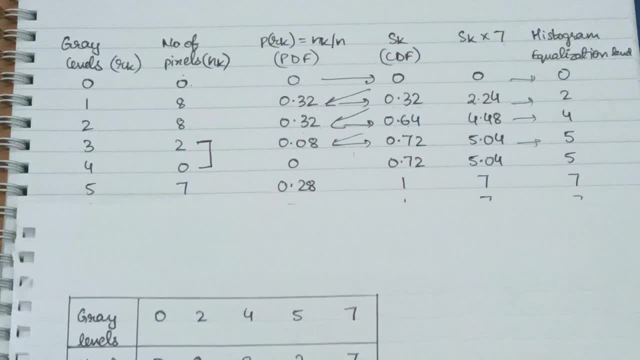 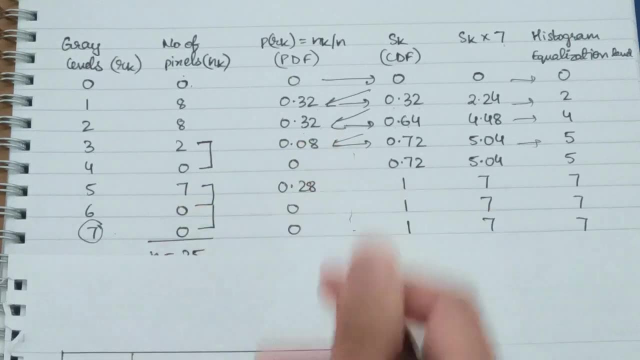 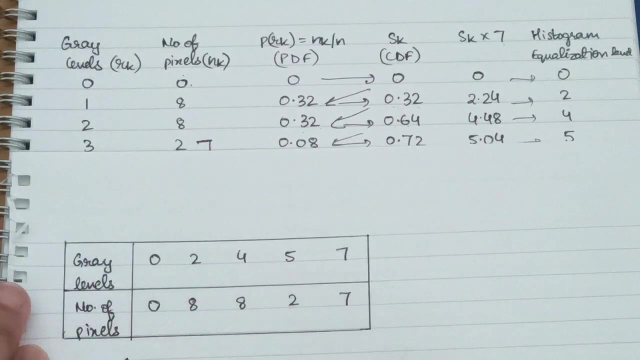 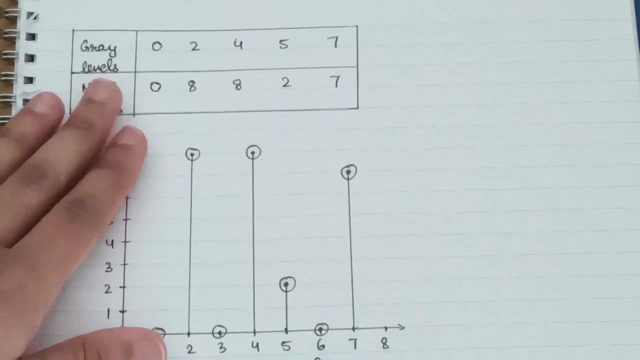 two values, okay, and then 7. if you see, 7 is 3 times. so we have taken the sum of these three values, which is nothing but 7. so based on those, we drew this table. and then, once we drew this table, based on these values, we drew our histogram. so if you see this, for 0 it is 0. for 1 also, it is 0 because 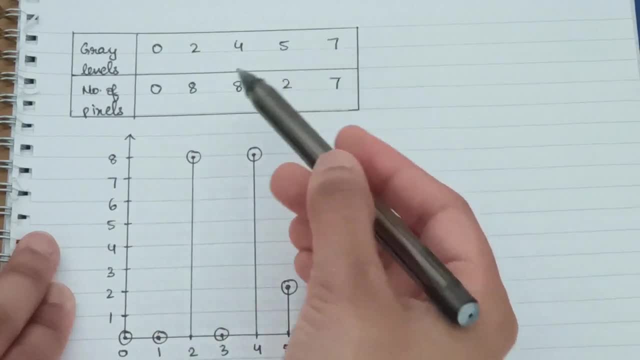 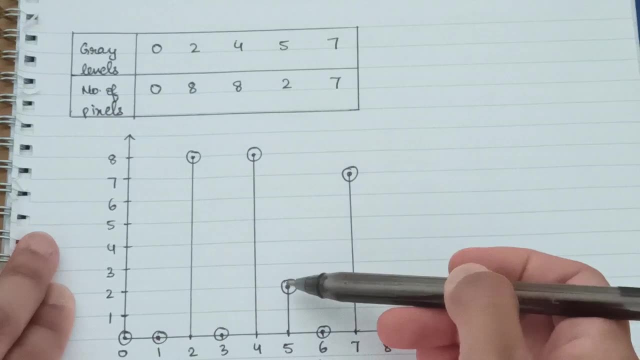 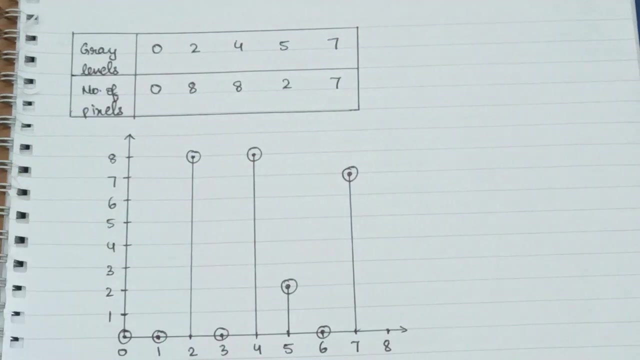 there is no 1 in our new grey level values. for 2 it is 8, for 4 it is 8. for 5 it is 2. so we have just drawn 2 and then for 7 it is 7. so this is our new processed histogram. 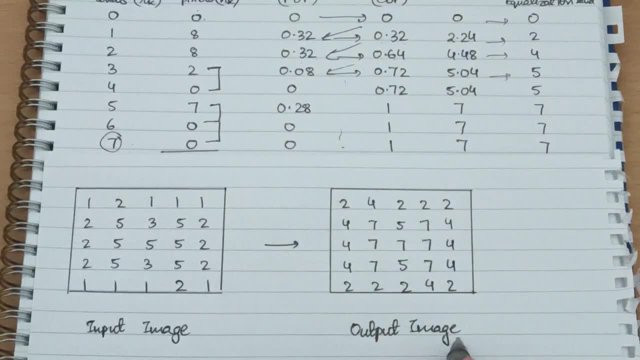 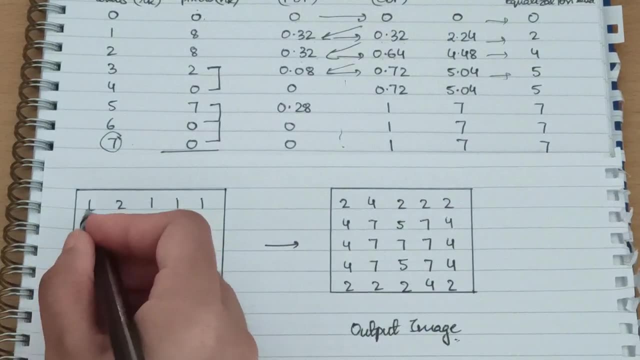 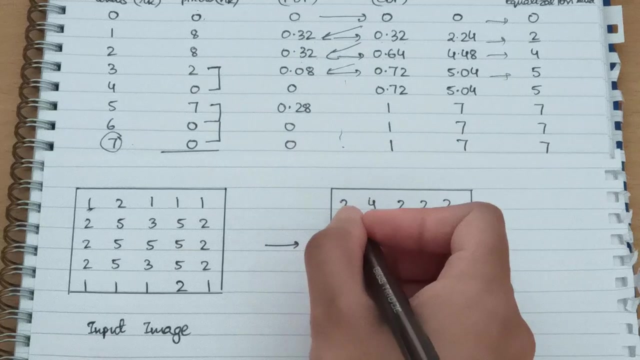 now for calculating the output image. what we did is we used the same table. ok, and now? the first value of the input image was 1, and 1 corresponded to the histogram equalization level of 2, so we have just substituted 2 here. we have written it down as 2. similarly, we 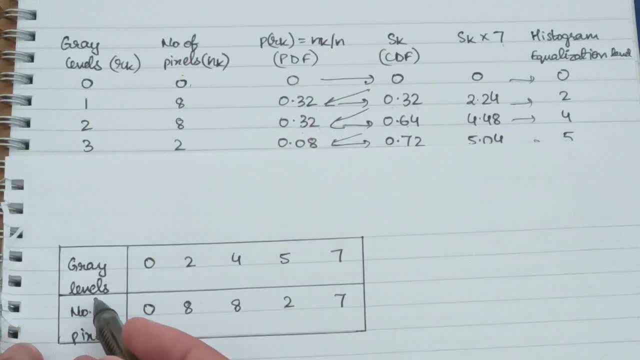 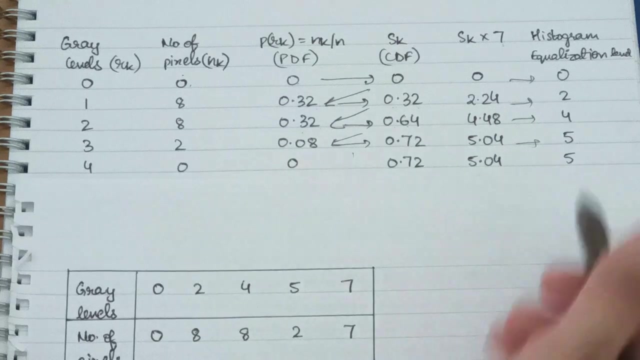 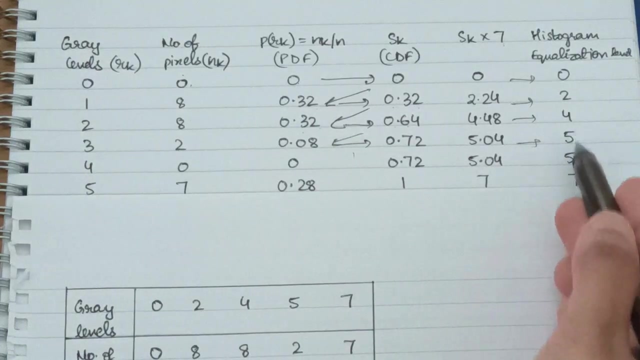 okay. here we have gray levels and number of pixels, the new gray levels. so this: these values are from the histogram. equalization levels: 0- we've just written it here. 2- we have written it here. 4- we have written it here. okay. 5- now what happened is that 5 was twice okay over here. we just wrote it. 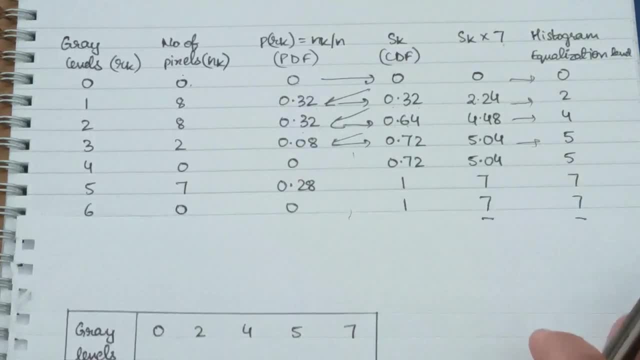 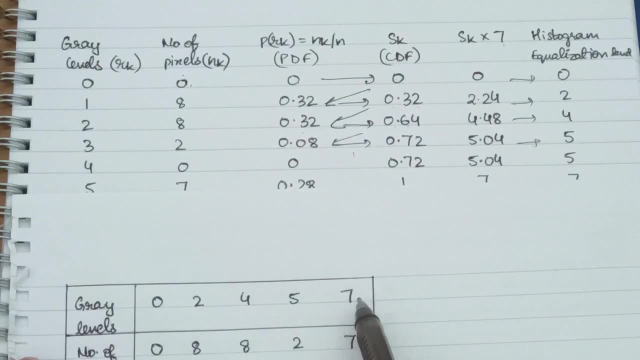 once, and similarly, 7 was thrice, if you see this. so we have that too. we have just written down once, and then we have written the corresponding number of pixels. for 0, it was 0. for 2, it was 8. for 4, it was 8 for 5, since 5 was 2 times. 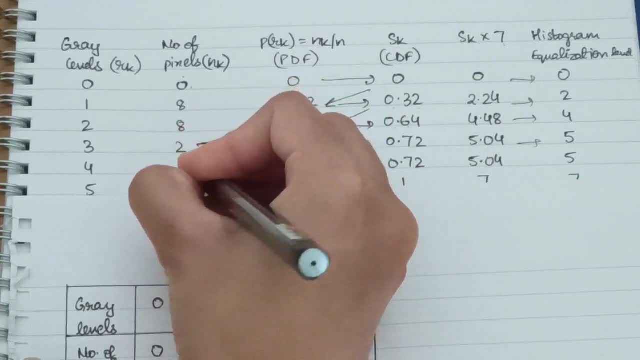 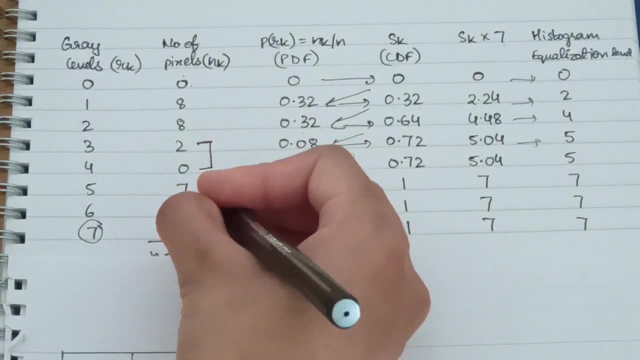 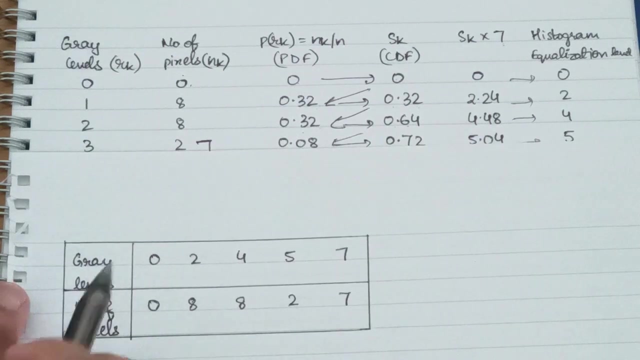 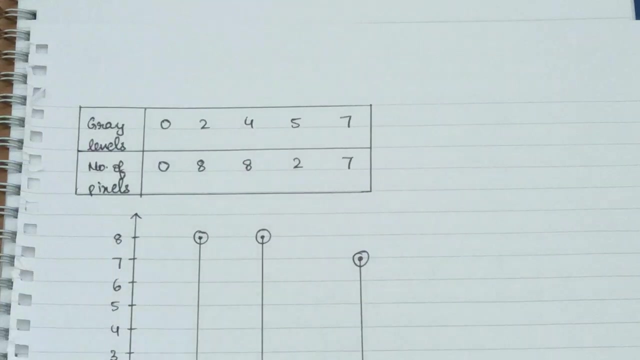 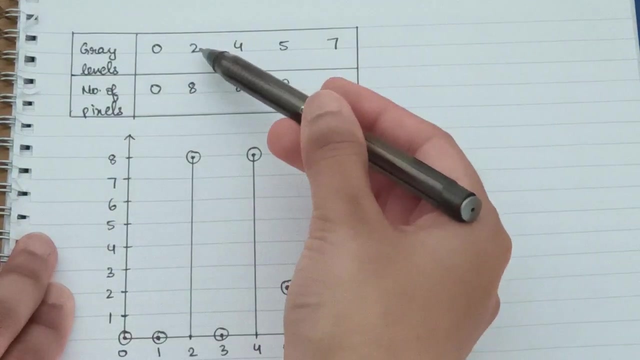 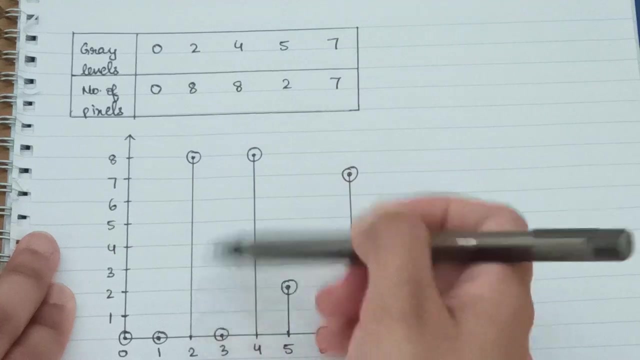 so we took the sum of these two values, okay, and then 7. if you see, 7 is 3 times. so we have taken the sum of these three values, which is nothing but 7. so, based on those, we drew this table. and then, once we do this table based on these values, we drew our histogram. so if you see this: for 0 it is 0. for 1 also it is 0 because there's no 1 in the new gray level values, for 2 it is 8. for 4, it is 8. for 5 it is 7. and then, once we drew this table based on these values, we drew our histogram. so if you see this, for 0 it is 0. for 1 also it is 0 because there's no 1 in the new gray level values for 2 it is 8. for 4 it is 8. for 5 it is 7. and then, once we drew this table based on these values, we drew our histogram. so if you see this, for 0 it is 0. for 1 also it is 0 because there's no 1 in the new gray level values for 2 it is 8, for 4 it is 8, for 5, it is 8, for 5 it is 7. and then, once we drew this table based on these values we drew our histogram. so if you see this for 0, it is 0. for 1 also it is 0 because 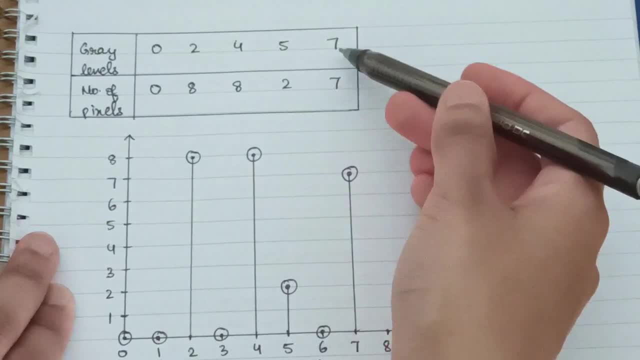 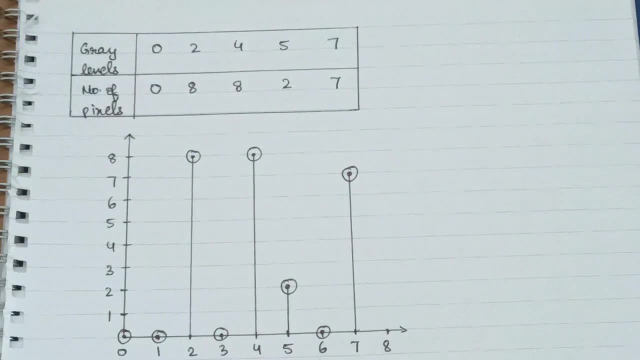 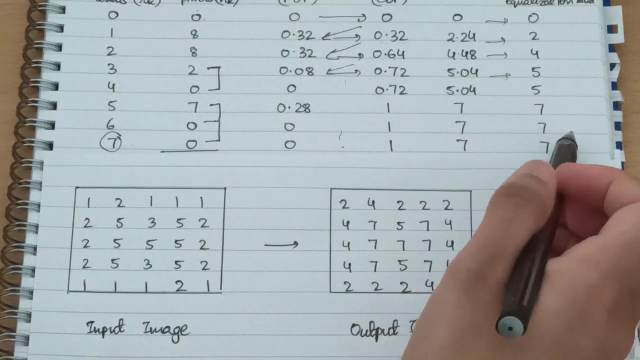 is 2, so we've just drawn 2, and then for 7, it is 7. so this is our new processed histogram. now for calculating the output image. what we did is we used the same table, okay, and now the first value of the input image was 1, and 1 corresponded to the histogram. 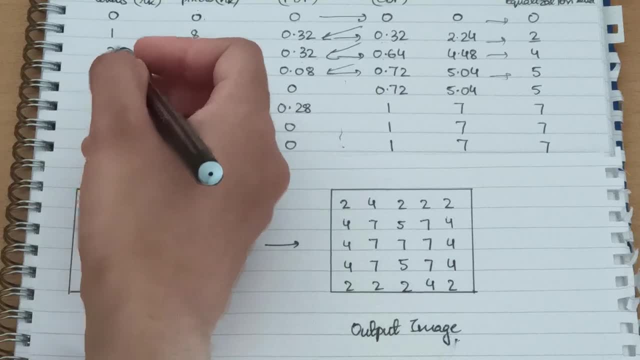 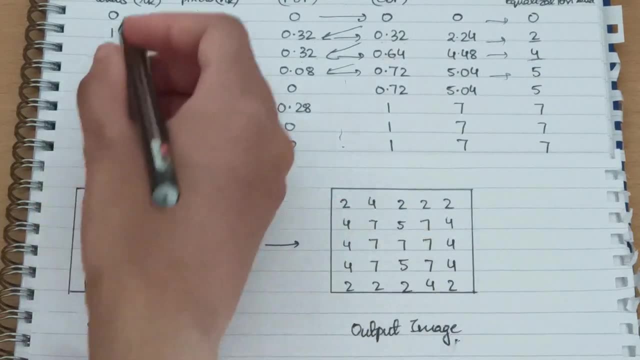 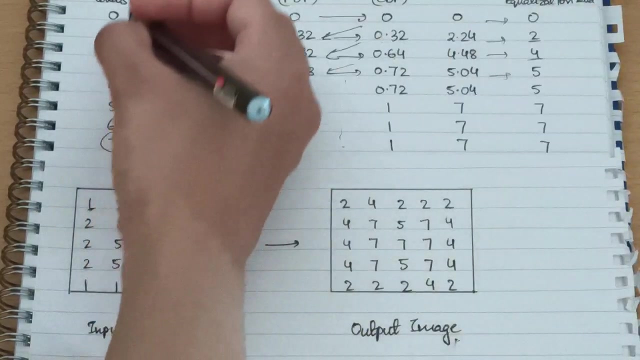 have written it down as 2, similarly 2. if we check in the grey levels, it is 4. the histogram equalization level is 4 for it. so we have just substituted 4 for 1. the answer is again 2. so we have substituted 2. so, based on these values, the first column and the last column. 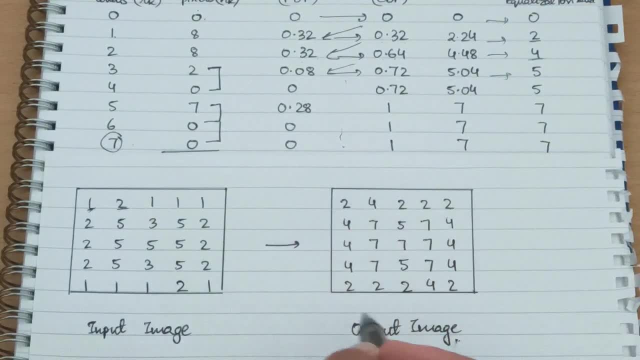 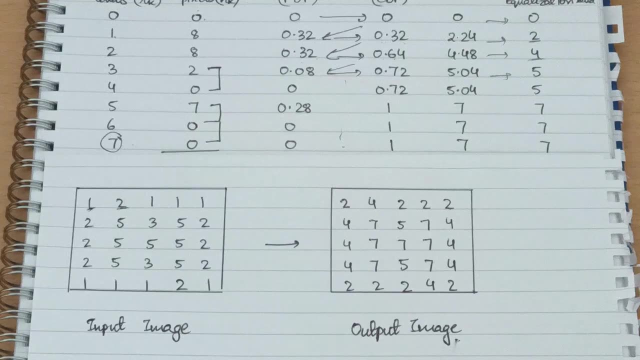 we have filled up our output image, so this comes out to be our final output image, and that's it for the lecture. i will see you in the next one, thank you. 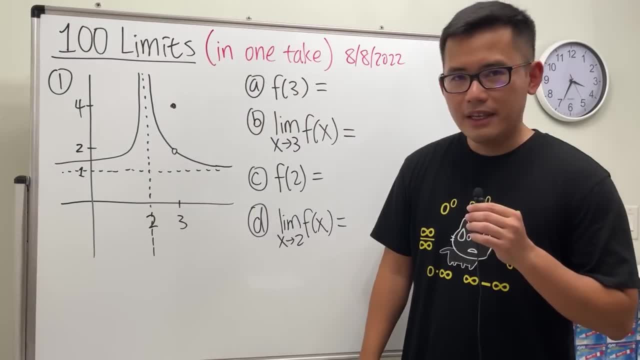 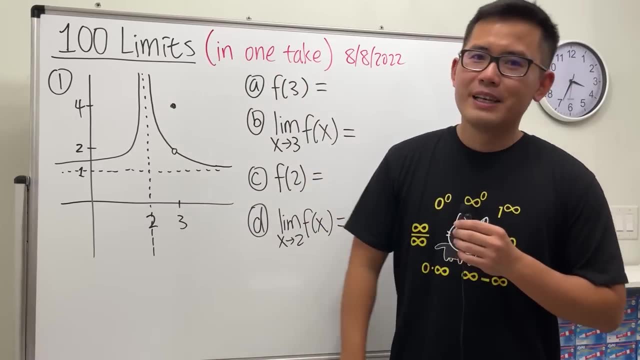 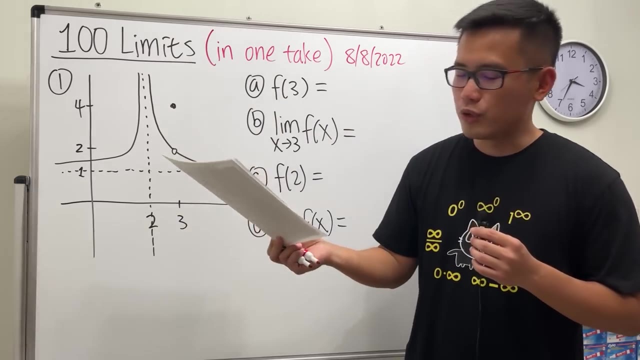 Yes, I'm serious. Today we'll be doing 100 limits and of course, we'll be doing them in one take. I know finally right, And you know the deal. The file is in the description for your good convenience already, so go ahead and download them and work out the questions. 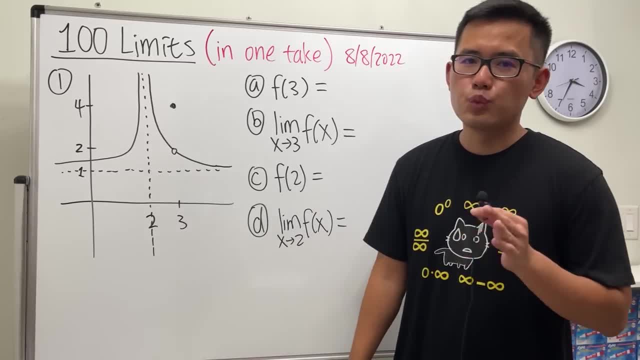 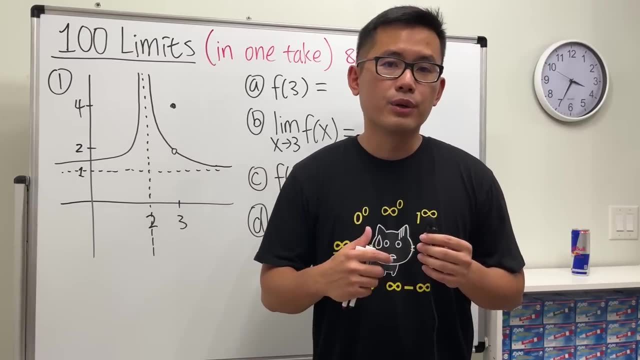 along the way, We will cover everything that you have to know for Calculus 1 and Calculus 2, including how to determine the limits from the graph and then how to do the algebraic limits and also the definition of derivatives, L'Hopital's rule, and we'll also talk about 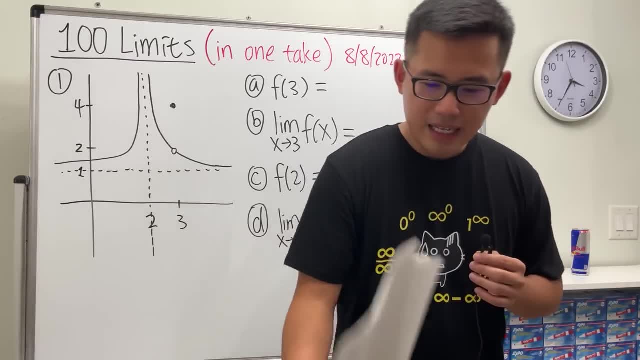 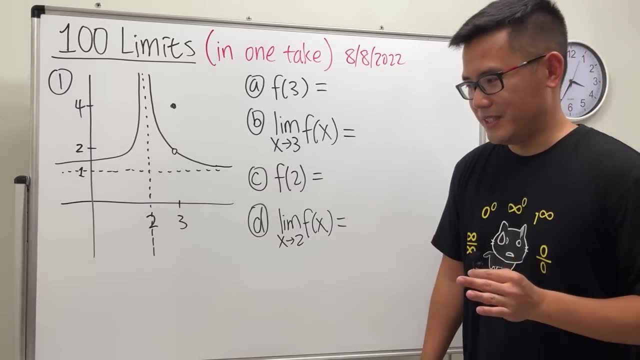 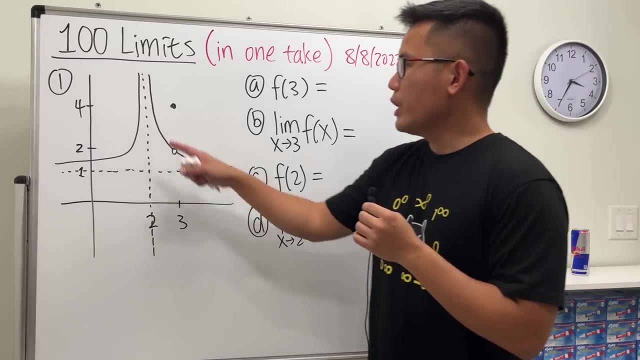 the epsilon-delta definition and also, yeah, this kind of very long limits at the very end. So, yep, you're going to have tons to learn in this video. I don't know how long it's going to take, but let's just go ahead and get started. Here we go, So we're given. 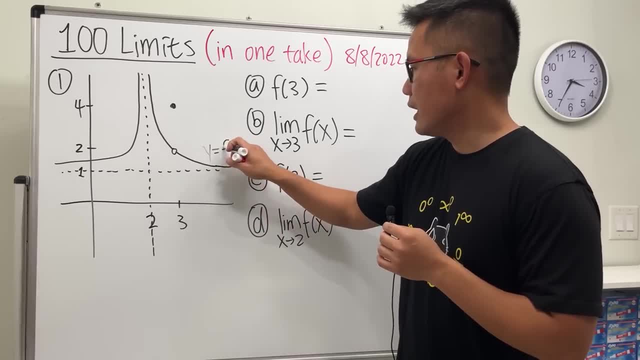 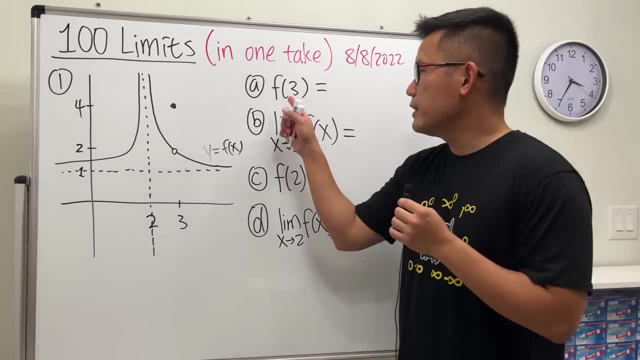 the graph of the function. so this right here is just going to be: y is equal to f of x, and then you can see a better picture on the file. Seriously, look at the PDF. All right, so first off, we are going to find the value. 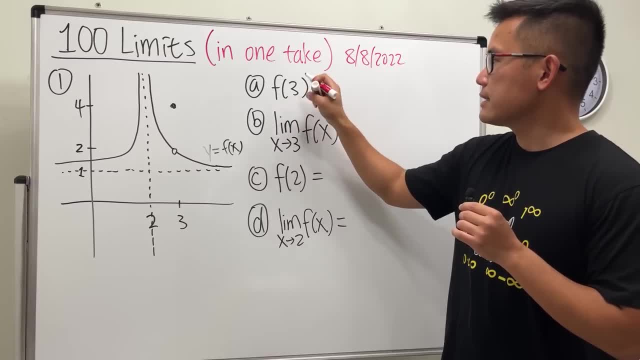 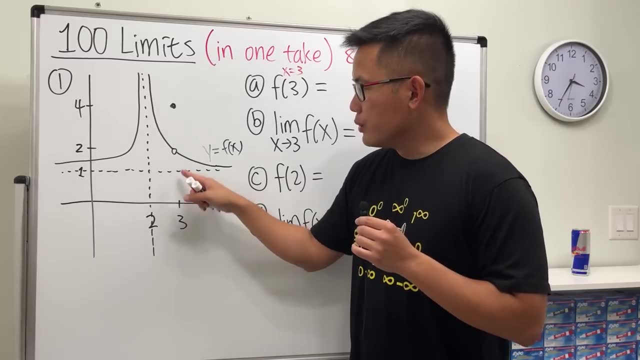 for f of 3.. So the way to read this is that x is exactly equal to 3.. This is not a limit question, So we go to: x is exactly 3.. Do not look at the open circle, but rather you have.